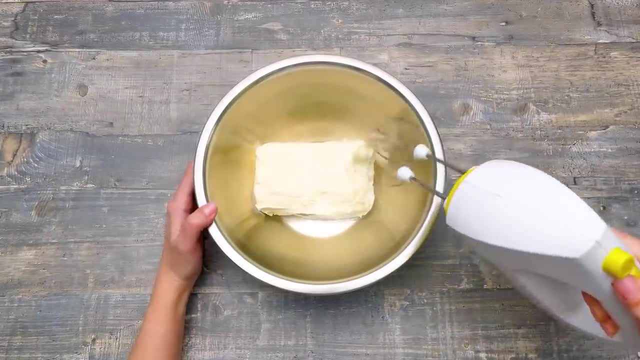 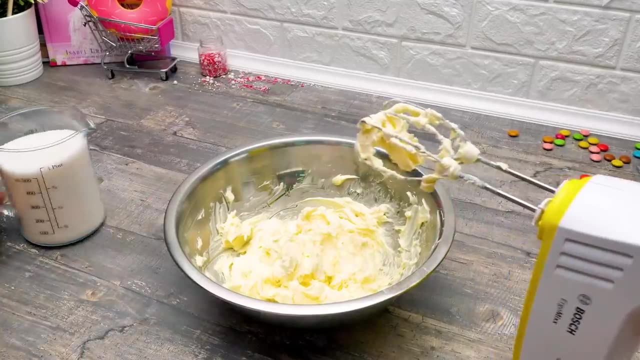 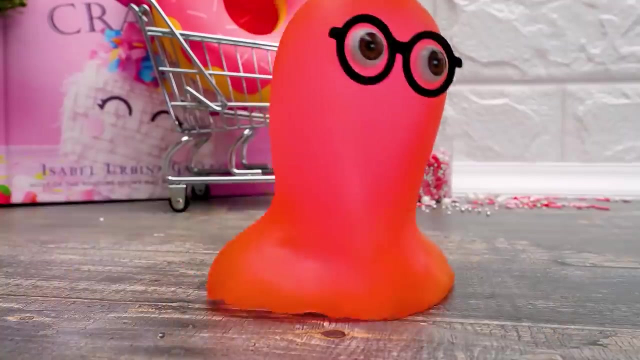 Now let's beat the butter to make it creamy. Don't forget about the sugar, Sue. I like it sweet. Here we go. Beat it for 6-8 minutes on a medium or high speed. Ready Start One and two and three. 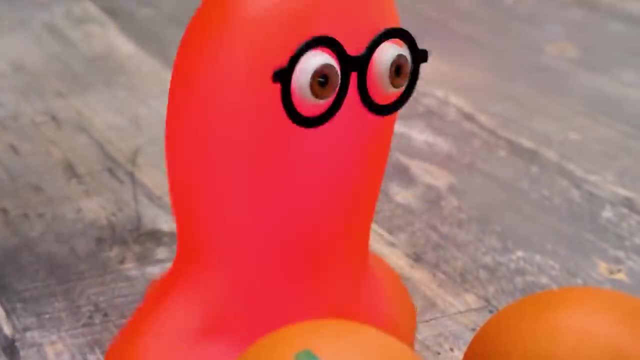 Cheddar, me cheddars. It's a whole bunch of them. We'll add eggs to the batter one by one And continue mixing. The main point is not to stop. Our unicorn cake will be so fluffy and creamy. I can't wait to taste it. 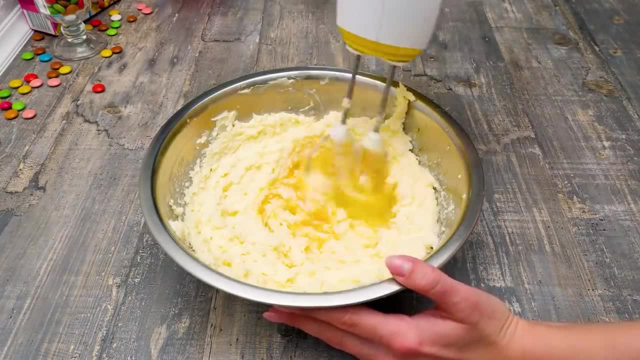 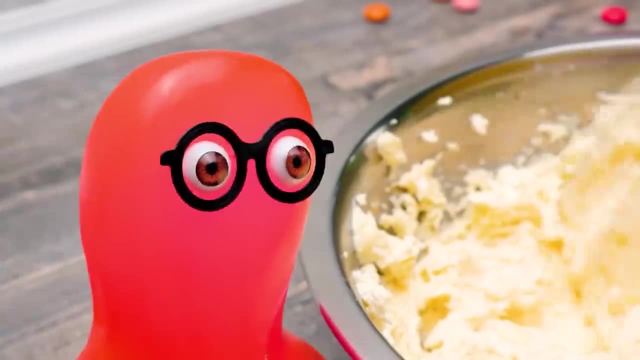 Be patient, Sammy. Let's add some vanilla extract for a nice smell, And then we'll add the food coloring. I'm gonna add some vanilla extract to the batter And then we'll add the sugar, And then we'll add the flour. 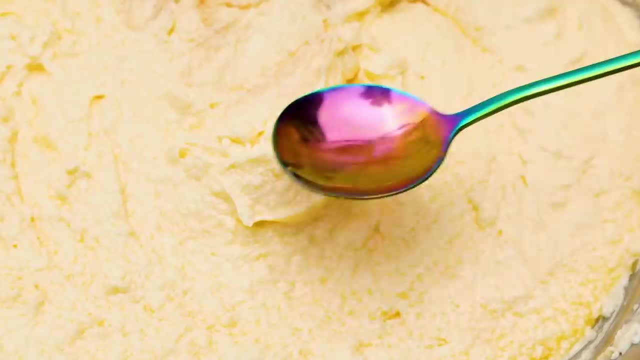 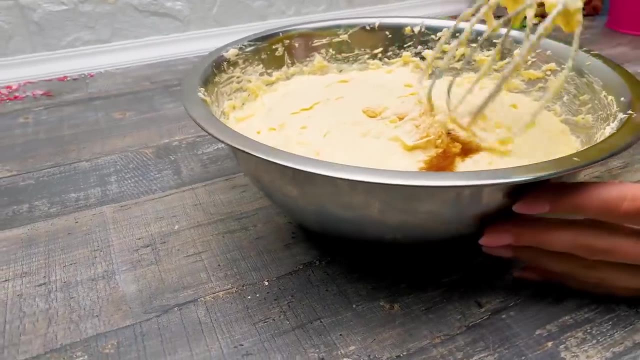 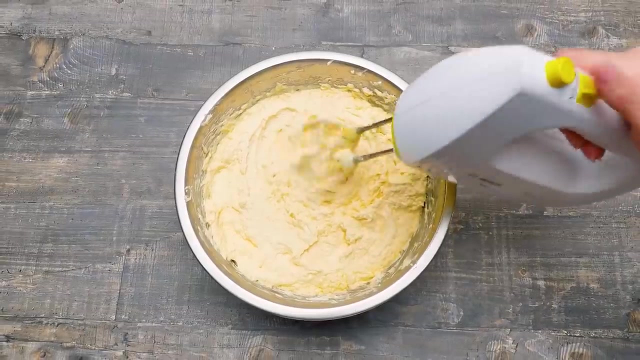 And then we'll add the sugar, And then we'll add the flour, And then we'll add the sugar, And then we'll add the vanilla extract for a nice smell and taste And more mixing, And finally the flour. By the way, Sammy, when is National Unicorn Day celebrated? 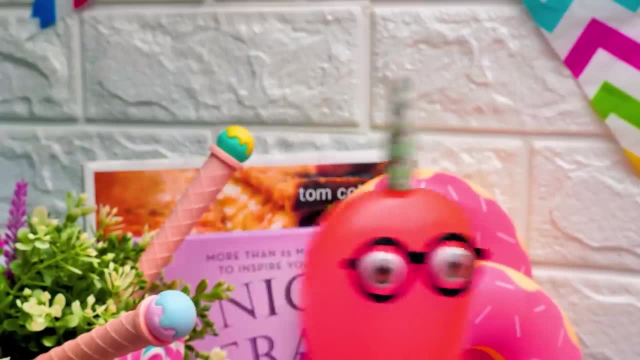 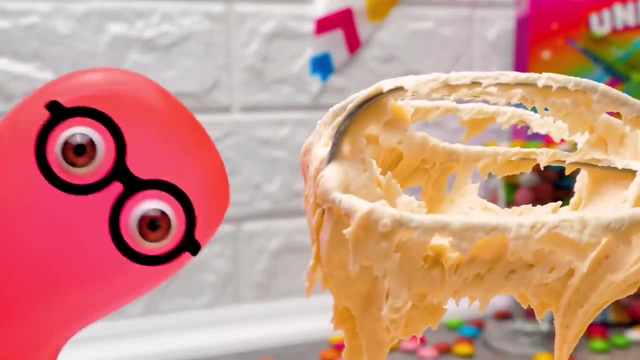 On the 9th of April, And that'll be the first slime unicorn in history, And the slickest one. Well, every unicorn is precious. Mmm, It smells so nice, Can I try it? Mmm, It smells so nice, Can I try it? 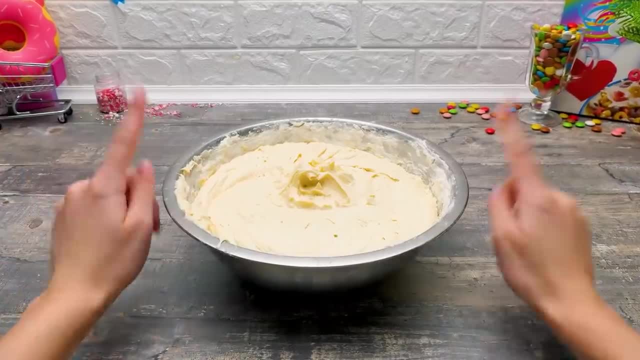 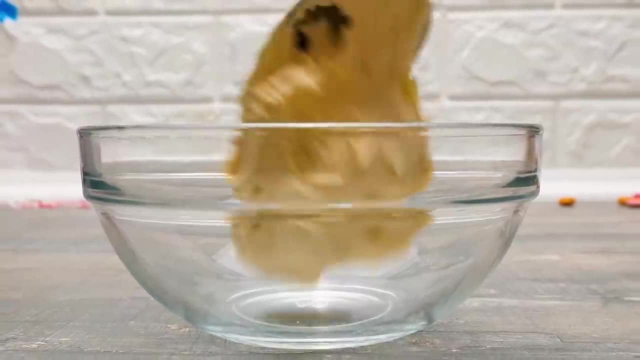 Hold it. sweet tooth. I know you'll eat it all if you can. I know you'll eat it all if you can. Now we need to divide the batter. Now we need to divide the batter into six parts, But I agree, it looks really yummy. 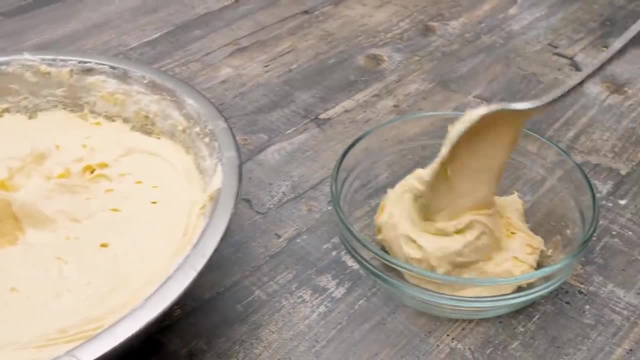 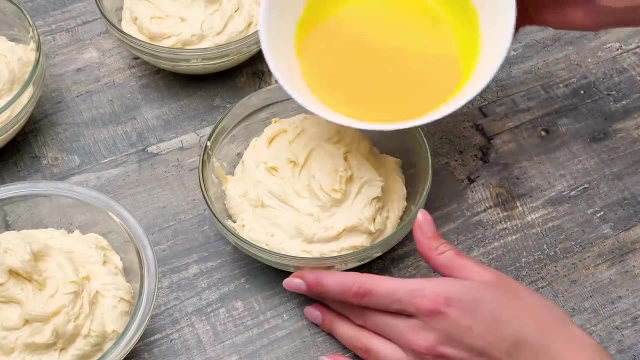 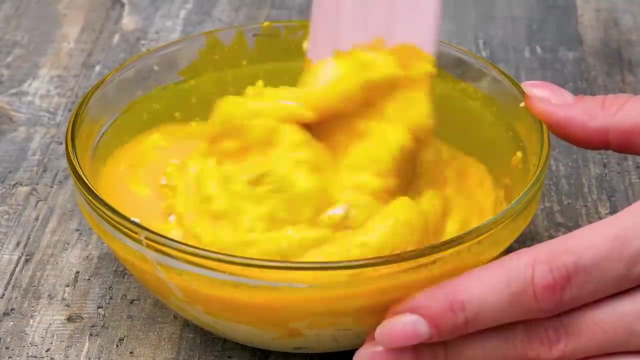 But I agree, it looks really yummy. Uh-oh, They all look the same. How do we know which one is where? We'll color them? of course We'll create a rainbow. We'll create a rainbow. We'll create a rainbow. 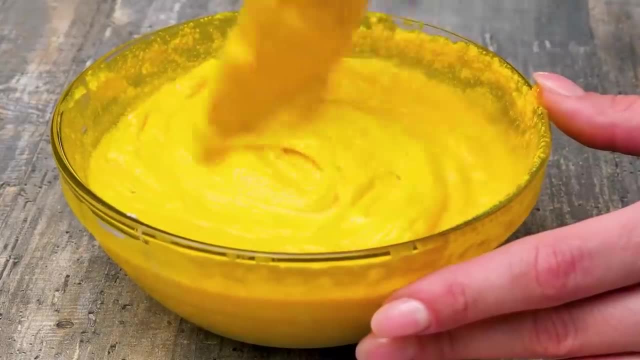 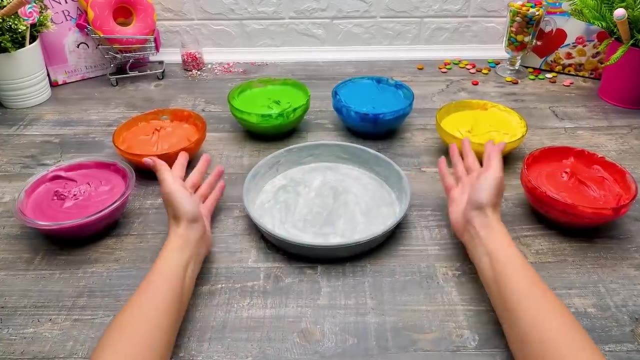 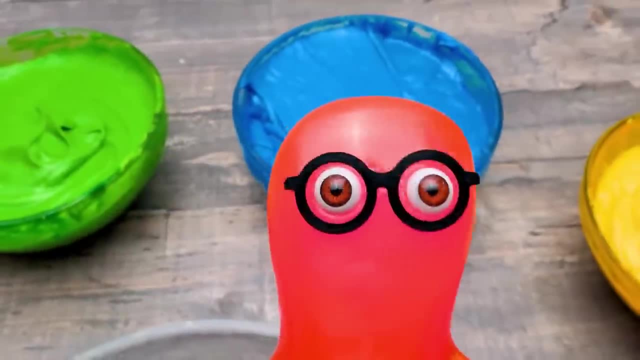 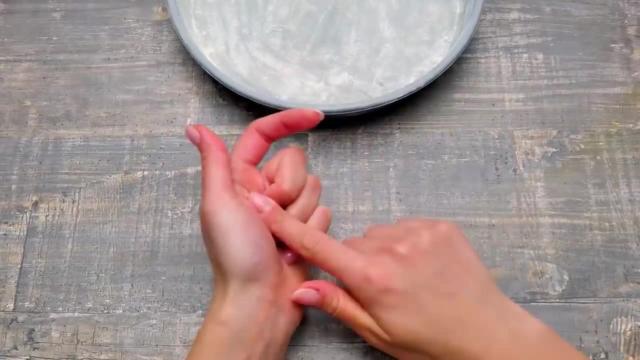 Oh, it's so hard. Maybe blue- I like blue, No, green is better. I'll count to three. One, two, three, One, two, three. Okay, I picked this one. You're so impatient, Sue. 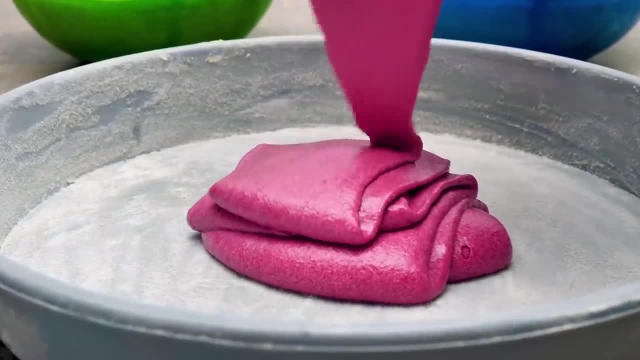 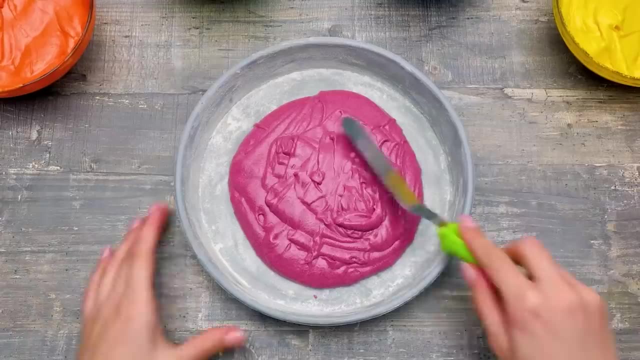 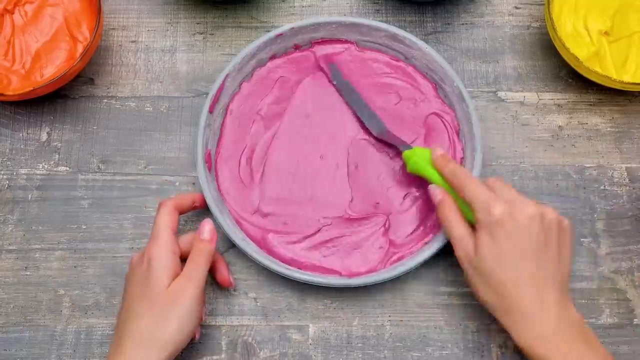 Well, I knew otherwise, you'd be choosing for ages. Well, I knew otherwise, you'd be choosing for ages. Let's spread the batter inside the baking pan. Let's spread the batter inside the baking pan. Whoosh, Whoosh. It should look smooth and even on the surface. 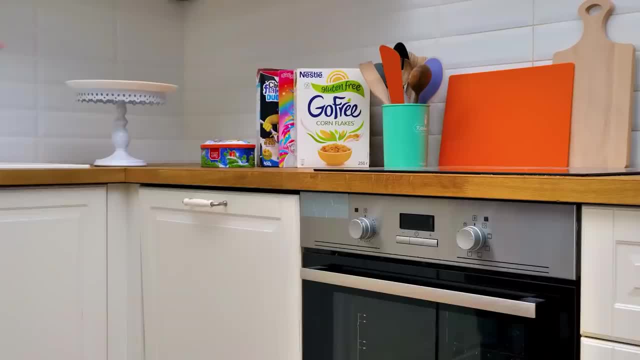 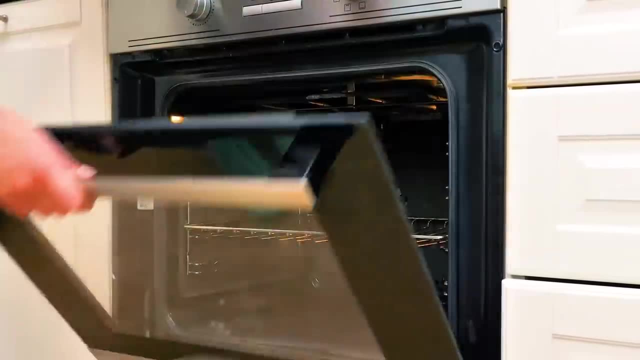 It should look smooth and even on the surface, Like this: Let's heat the oven to 170 degrees. Let's heat the oven to 170 degrees To bake our colorful cake layers. We'll send each of them to the oven for 18 to 20 minutes. 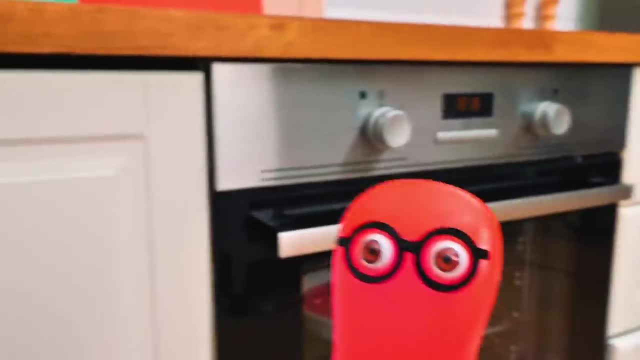 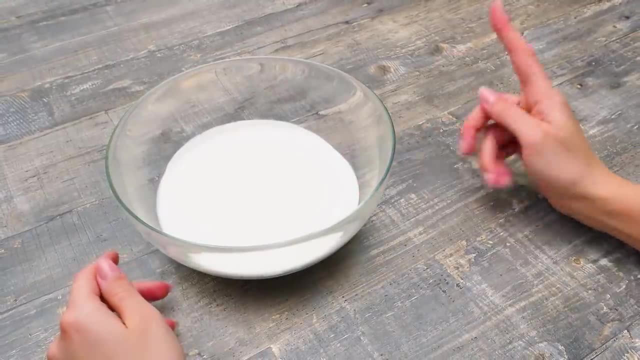 We'll send each of them to the oven for 18 to 20 minutes. Wanna see all the colorful layers together. Wanna see all the colorful layers together. Stay tuned: While the cake layers are baking and cooling down, Let's make a delicious frosting from cold heavy cream. 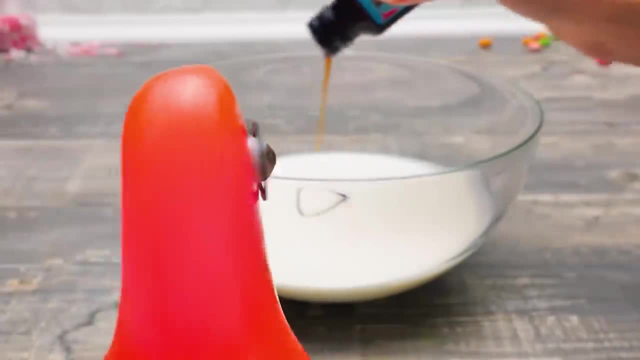 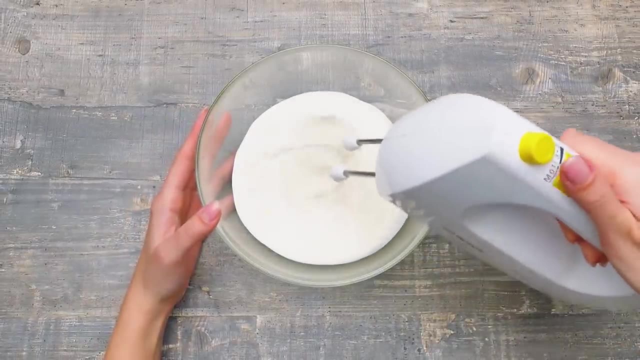 Let's make a delicious frosting from cold heavy cream. Our unicorn cake will smell like vanilla- So good I think it's a perfect smell for it. Guys, give a thumbs up if you agree. Guys, give a thumbs up if you agree. 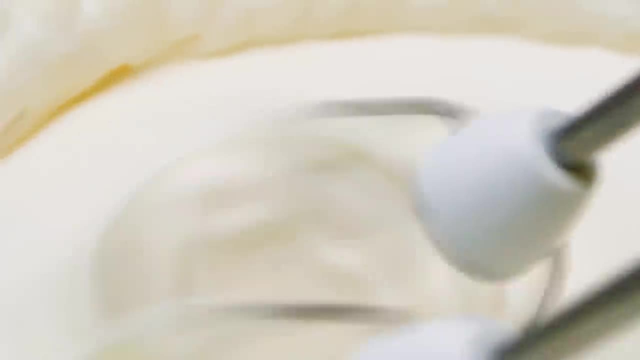 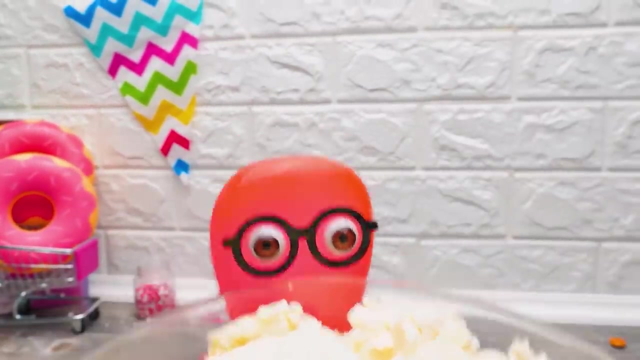 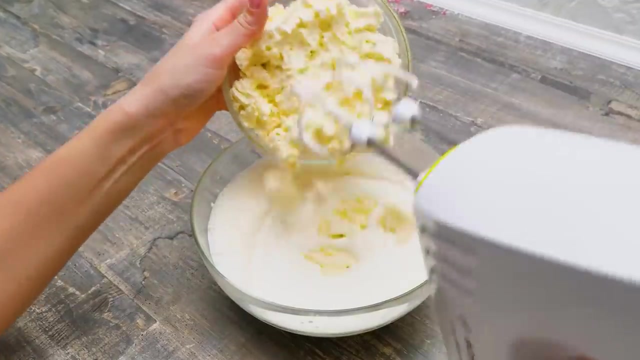 Swirl and whip, Swirl and whip Again and again, Again and again. Too much whipping will ruin our frosting. Too much whipping will ruin our frosting. Here in time. Heavy cream is ready. Let's add the cream cheese to it. 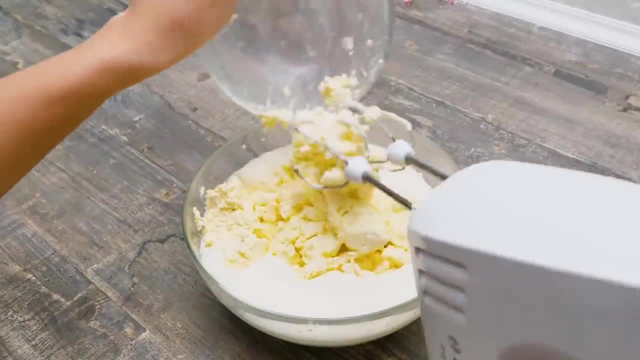 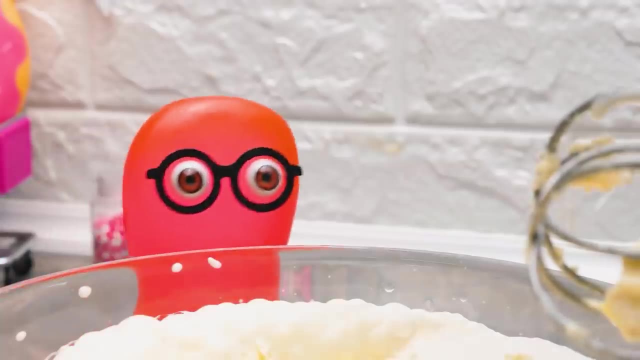 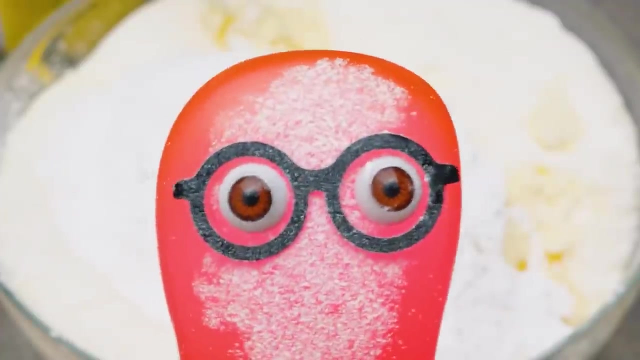 Let's add the cream cheese to it Like this, And some lemon juice- Squeeze harder, Squeeze harder. And some powdered sugar too. Our unicorn cake will taste like a candy. Our unicorn cake will taste like a candy. Now. you taste like a candy too, Sammy. 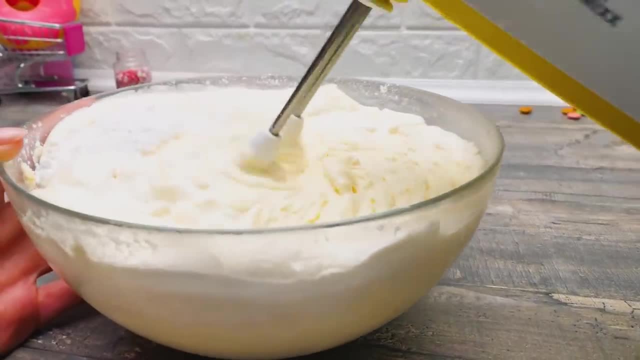 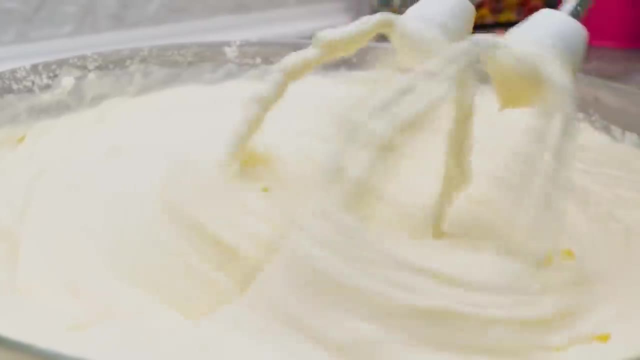 Now you taste like a candy too, Sammy. All the ingredients are in, so let's mix them well to make a smooth frosting. All the ingredients are in, so let's mix them well to make a smooth frosting. Phew, All cake layers are finished. 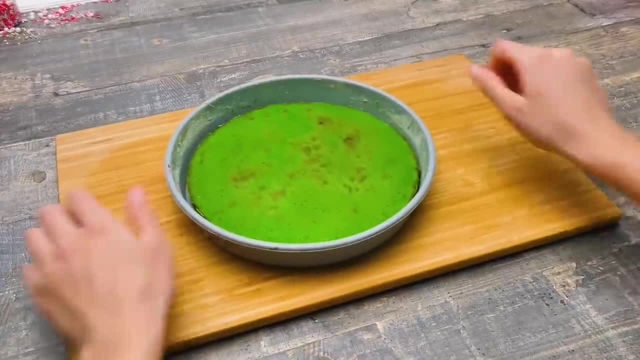 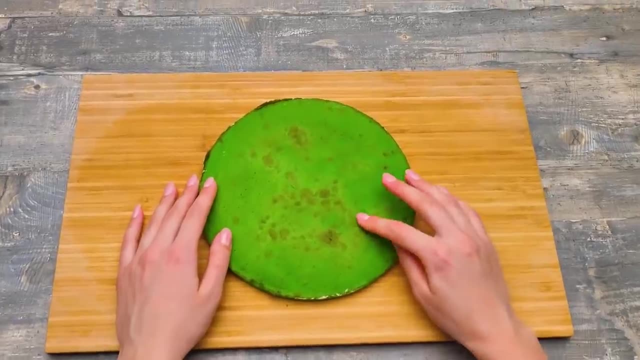 but they don't look good enough. Let's see, here's our green layer. Let's see, here's our green layer. Flip it over carefully. Ah, I got what you mean. Nothing to worry about, Sammy. Let's remove the brown crust and it'll be just right. 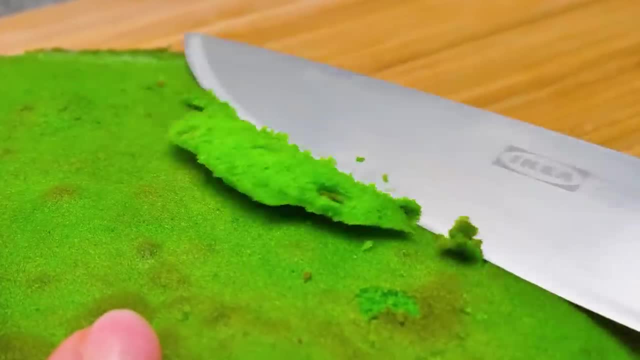 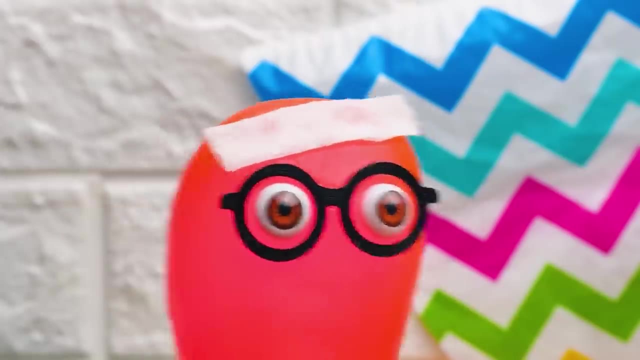 Let's remove the brown crust and it'll be just right. Phew, And I thought our party's ruined. You're a miracle, Susan. Check this out guys. We can already see fluffy and bright green sponge cake inside. We can already see fluffy and bright green sponge cake inside. 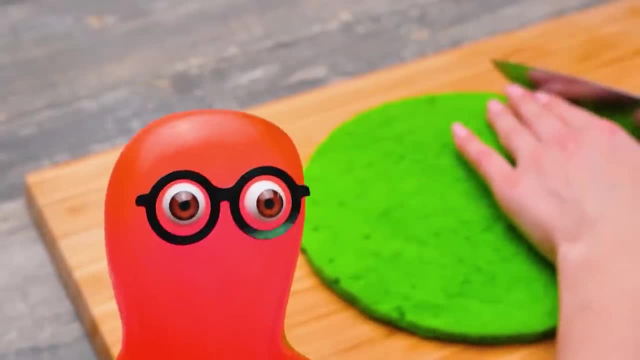 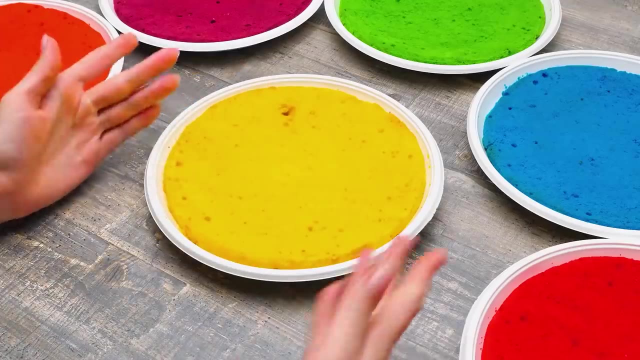 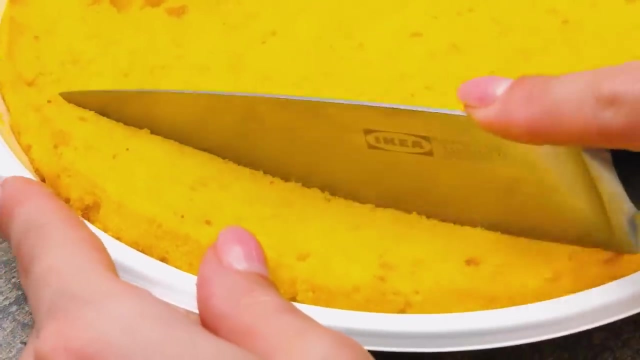 Guys, be careful with the knife. Better ask an adult to help you. Wow, It looks awesome. Now let's transform it to our liking. Now let's transform it to our liking. Let's cut out the left side. Use the knife carefully. 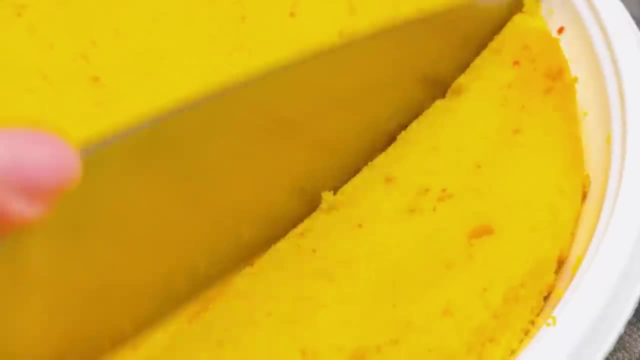 And the right side too, And the right side too, You'll get kind of a rectangular shape. Oh no, That's a waste of precious sponge cake, Susan. Oh no, That's a waste of precious sponge cake, Susan. 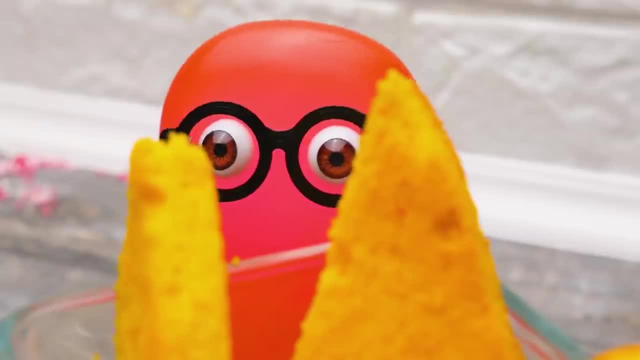 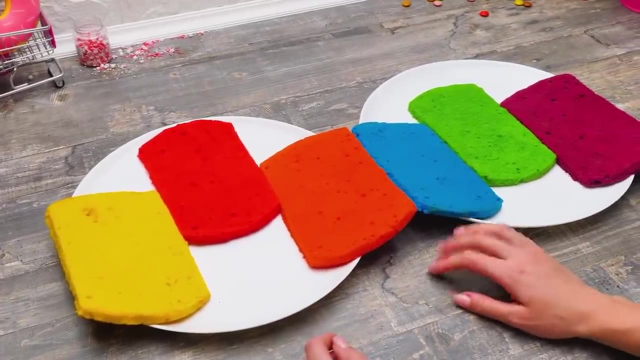 Then maybe you want to taste it. Now you're talking: I love sponge cake, Guys, this is what we've got after cutting everything out. Guys, this is what we've got after cutting everything out. What color should we start with? 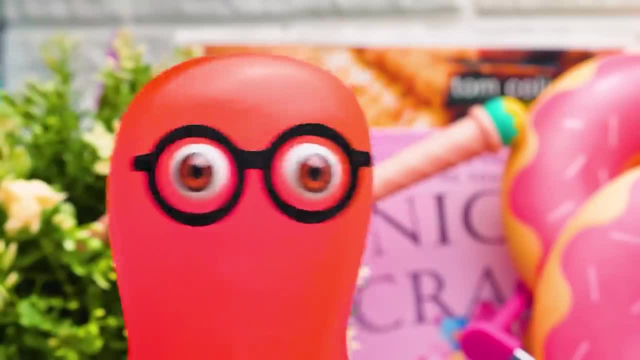 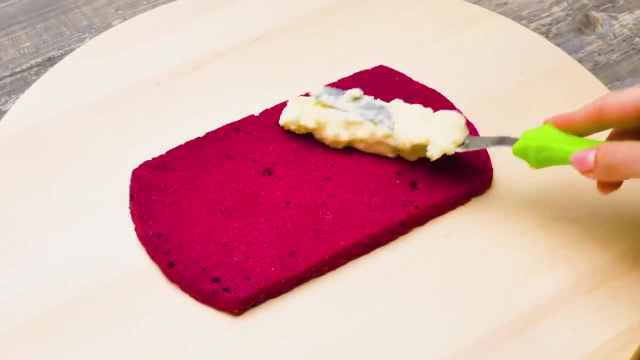 Just go with rainbow color order, Sue, big deal. Just go with rainbow color order, Sue, big deal. You're right, Sammy, We'll move from the bottom to the top. So the first one will be purple, And here is our white frosting layer. 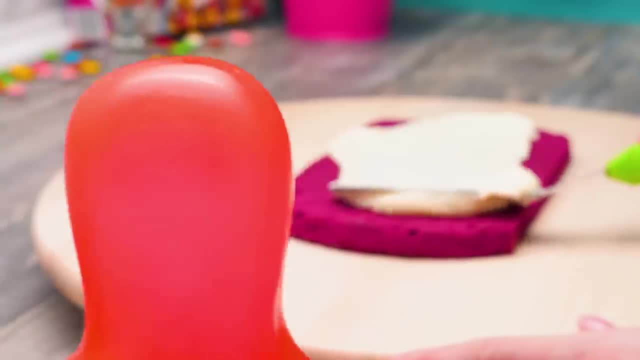 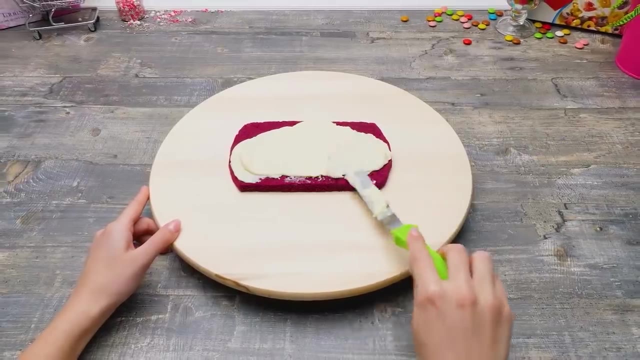 Looks so good. Don't be greedy, Susan. Add more frosting to the layer. Trust me, this amount is just enough. Trust me, this amount is just enough. Besides, we'll cover each layer with it, So let's use it wisely. 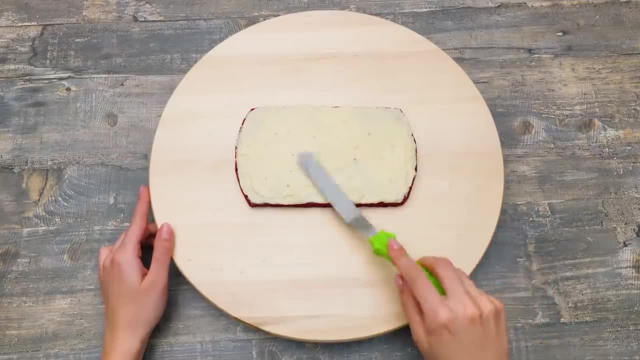 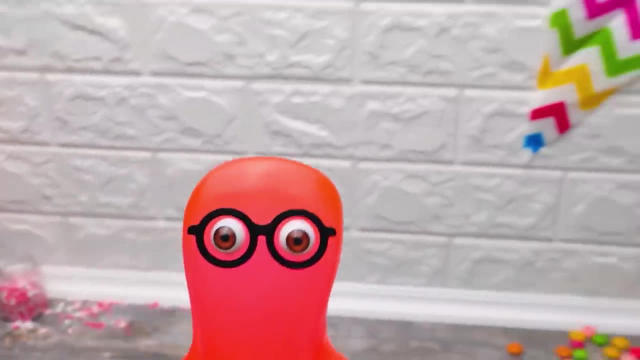 Oopsie, I won't taste it, or nothing will be left at all. The first frosting layer is finished And the next is blue. And the next is blue. Wait, What do you mean blue? Where is indigo Sammy? this cake rainbow has only six colors. 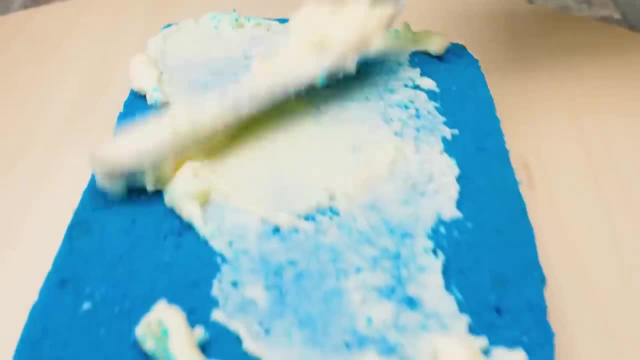 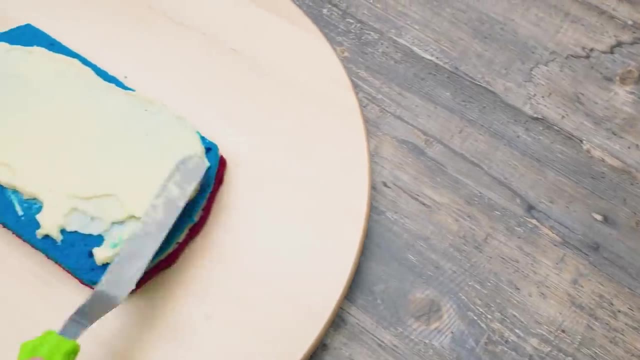 Sammy, this cake rainbow has only six colors. Let's let it be a unique one. Okay, it's unicorn day after all. It's unicorn day after all. Everything is possible. That's better. It'll be a perfect cake, I promise, But I need your help. 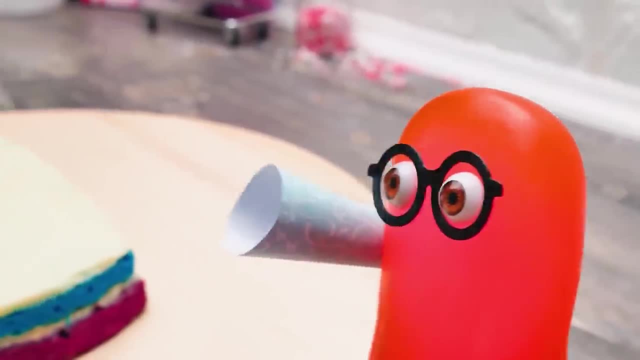 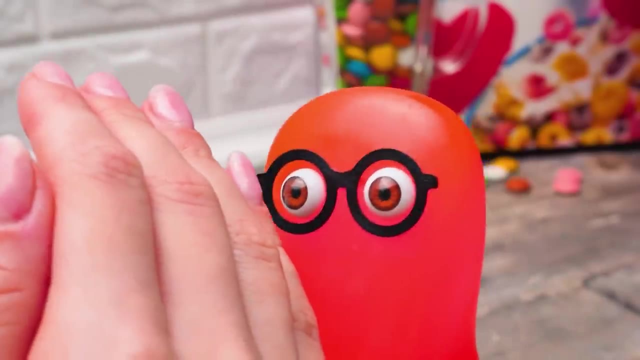 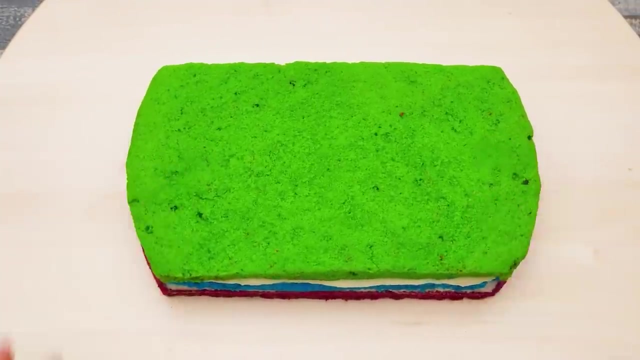 I'm ready. but whisper into my ear, Sue, It should say a secret. Okay, then I got it. Don't worry, It's gonna be perfect. Seems like Sammy will come back very soon, So I need to speed up too. 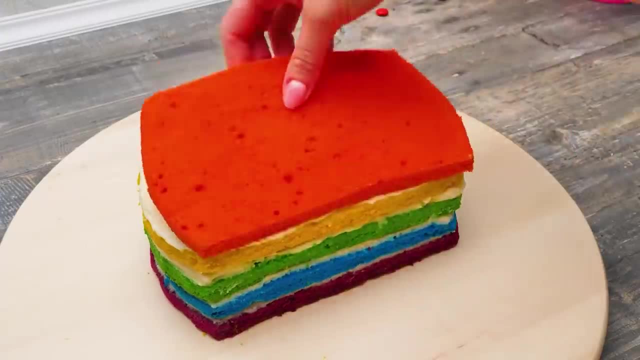 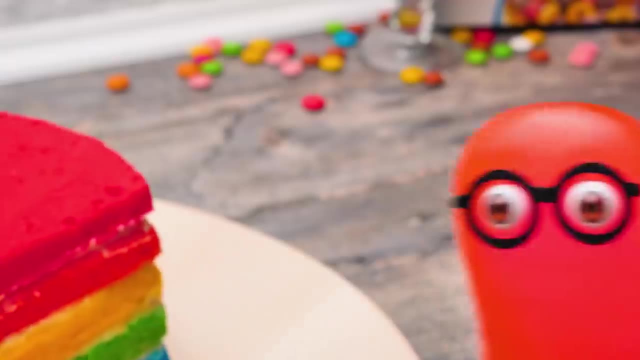 So I need to speed up too. Okay, we put all the layers in order. Okay, we put all the layers in order, but there's still some work to do And a big party's closer. now Let's continue. Let's give our cake a smoother shape. 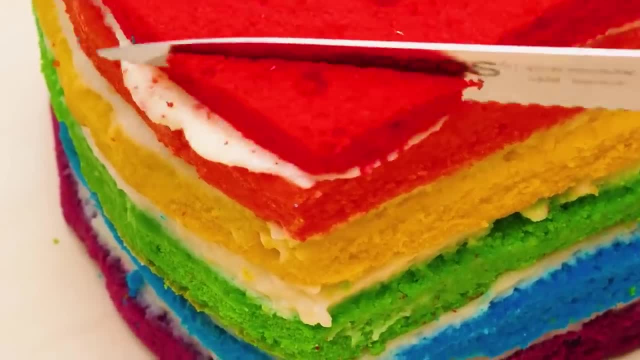 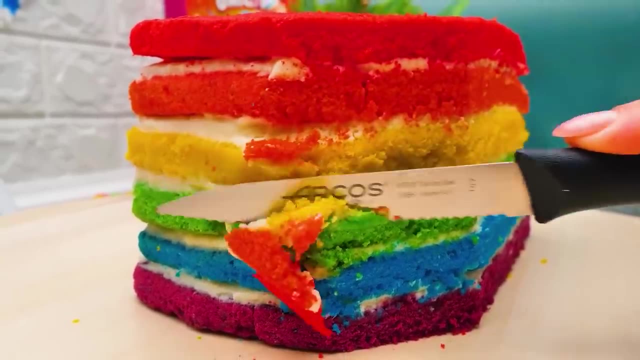 Let's give our cake a smoother shape. Cut off a small piece at an angle here, Cut off a small piece at an angle here And align the sides like this. Be careful while working with a knife guys. Be careful while working with a knife guys. 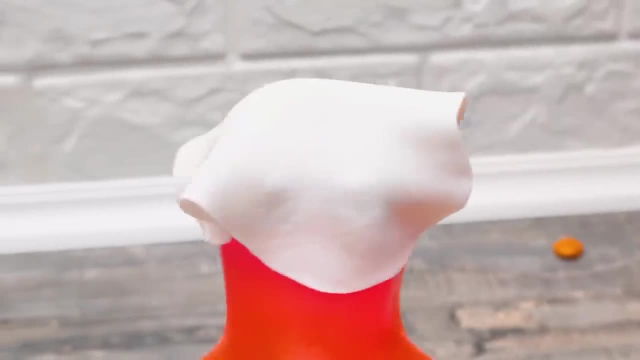 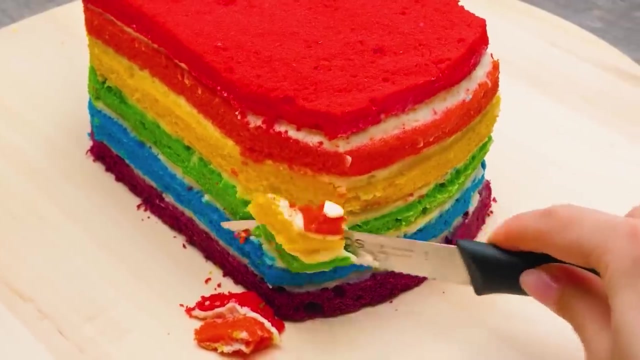 Oh, I can't see a thing. Sue, where's my work place? Go straight forward And after ten steps, turn to the right. Are you sure you don't need my help? Ha, Absolutely. I bought it to be a surprise. you'll see. 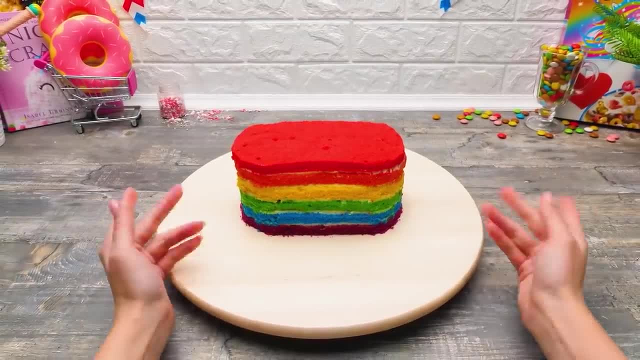 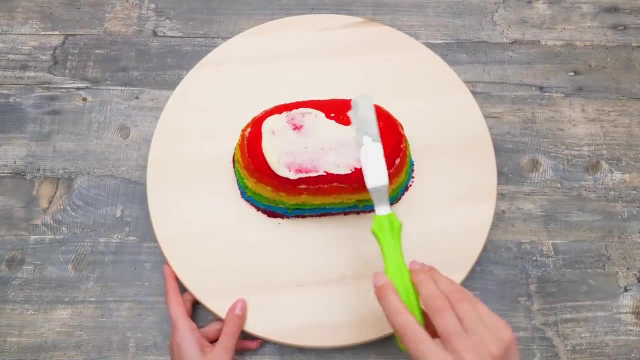 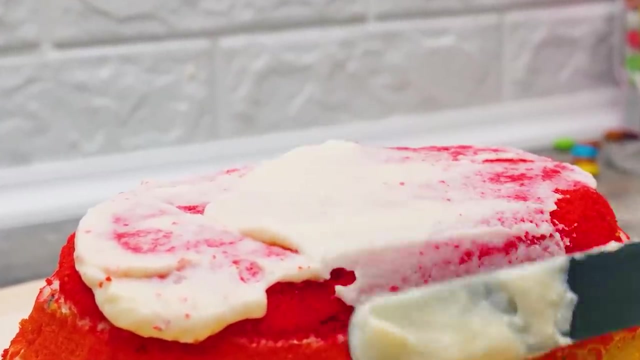 As this is a unicorn party, let's use some magic. Here we go, And this is the last frosting layer. Let's cover the cake with it. My mouth is watering. It looks so delicious. You can handle it. Susan Slimes can do it, and you can too. 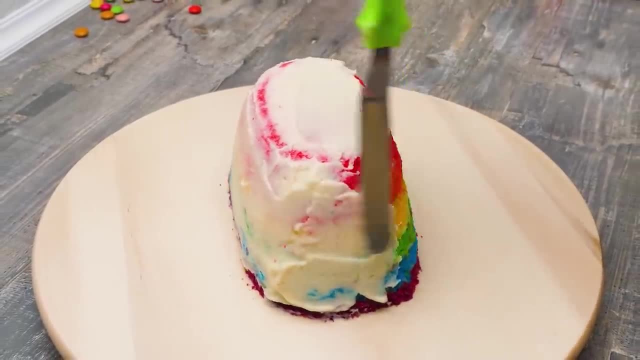 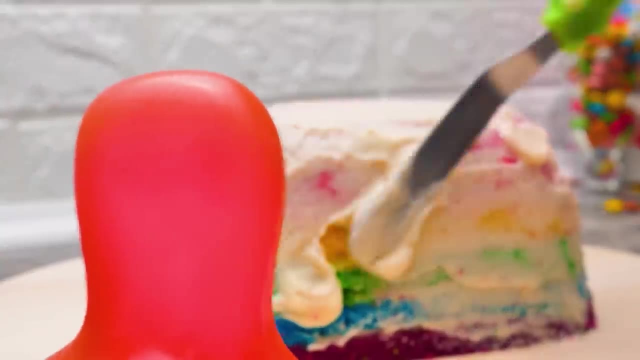 I'm trying, Sammy. By the way, did you finish it already? Did you doubt me? Of course I have, Really. Then can I take a look? Uh-uh, Don't get distracted, Sue, I'll show you at the right time. 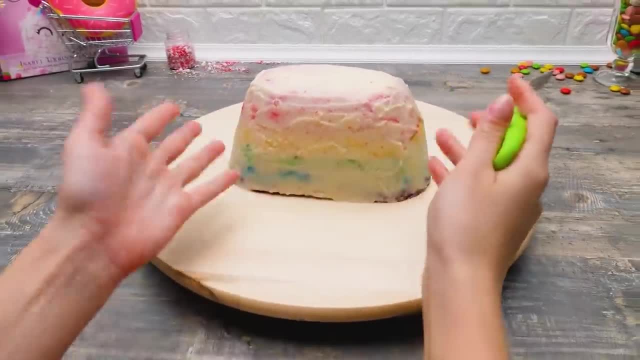 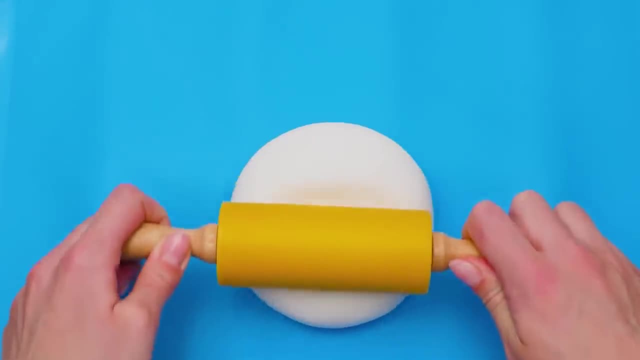 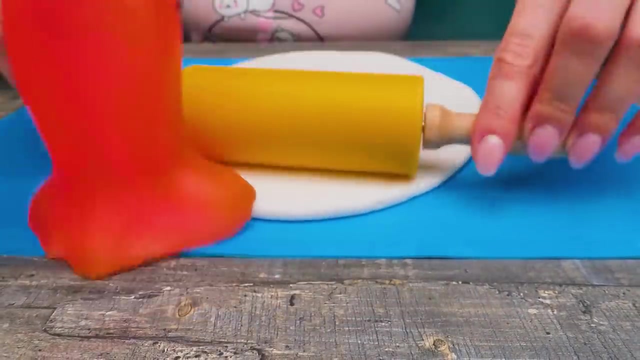 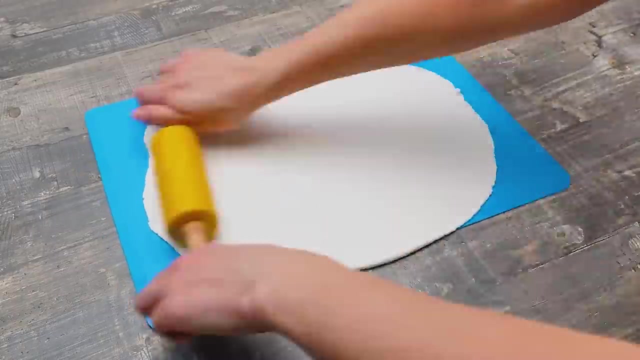 Mark your words, Guys. we're ready to start the decor part. We'll use white and colorful fondant for it. Let's roll it first and make a big round shape. Careful slime is on it's way. When the fondant is big and round enough, we'll cover our cake with it. 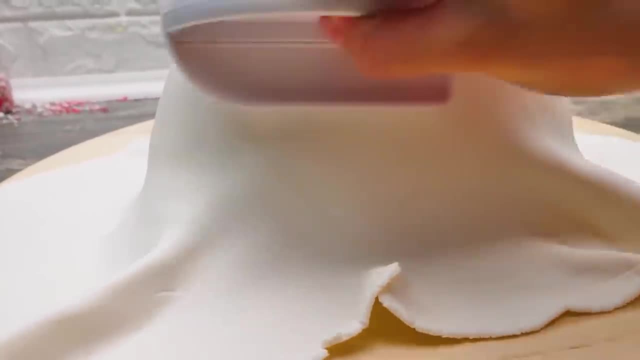 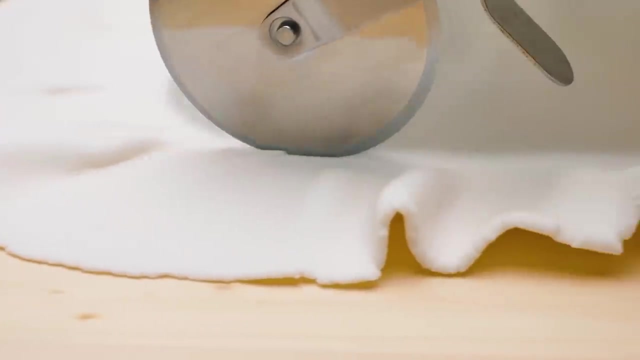 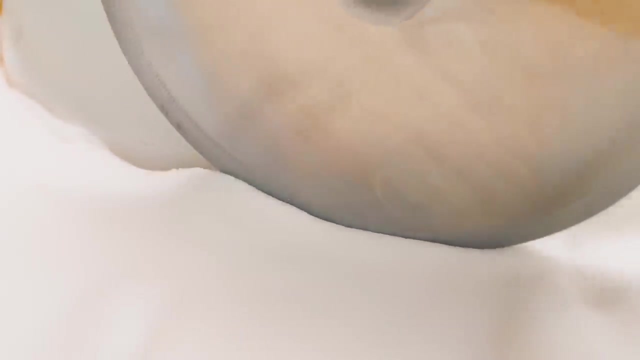 And smooth it out properly. No creases should be found. It looks like a thin blanket. Ha-ha-ha, Not anymore. We'll cut all the edges with a knife. Whoosh, Fast and clean. I'll prepare the cake for the next step. 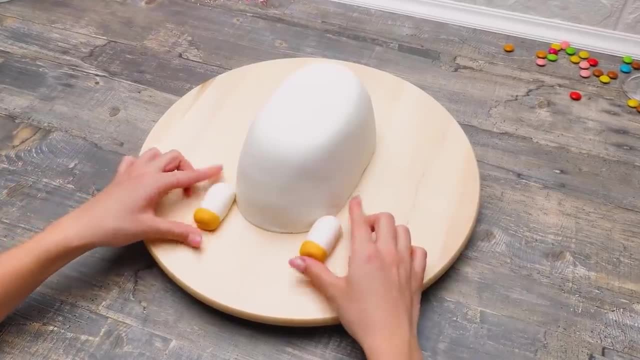 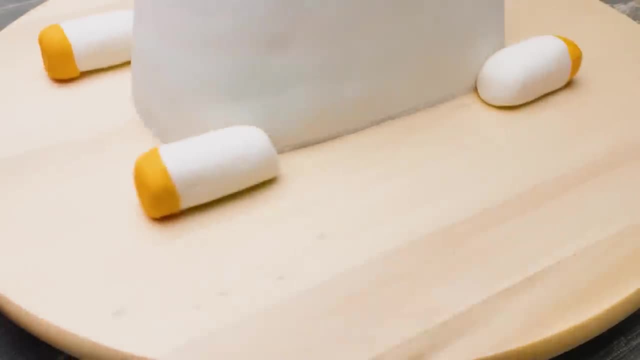 By the way, what will it be? Just add four pieces, Two to the front and two to the back. Do you recognize the shape? now I think it's time to bring my surprise. I'll be right back, Guys, check it out. 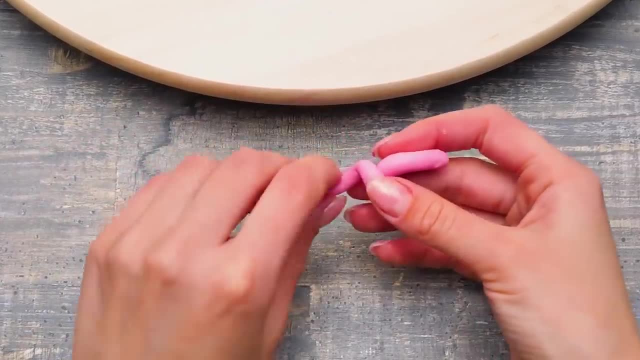 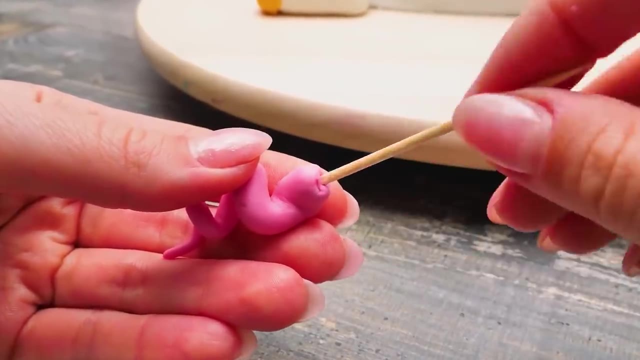 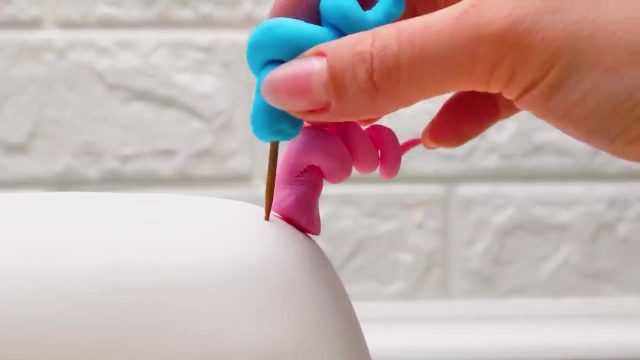 This pastel pink Looks amazing. Let's curl it- It's so adorable- And insert a toothpick to attach it to the cake. Here's a tail with pastel pink And blue. How lovely, Sue. it's time. 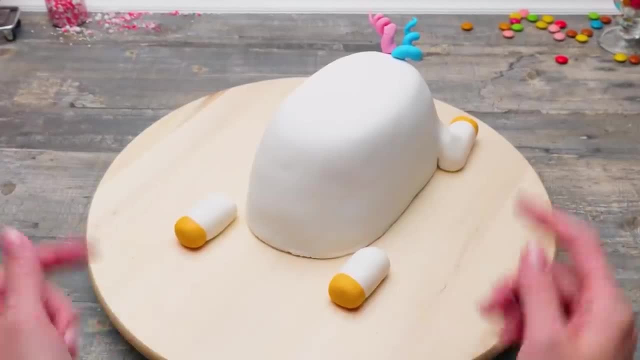 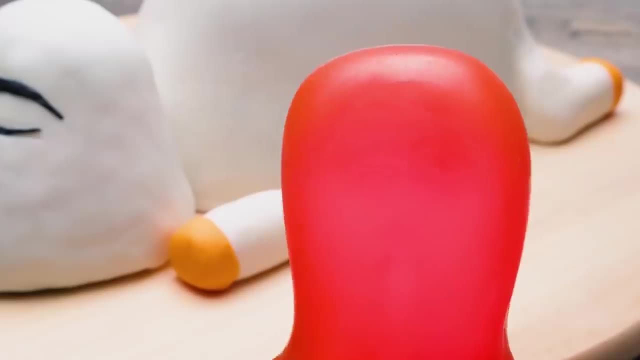 Can you close your eyes? Okay, but only for three seconds. Ready, Three Ta-da, Another six cake and frosting layers, Then fondant and my surprises: Are you ready? But I was in such a hurry that I missed a few details. 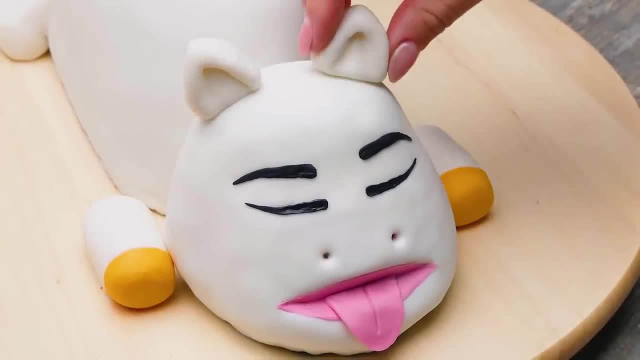 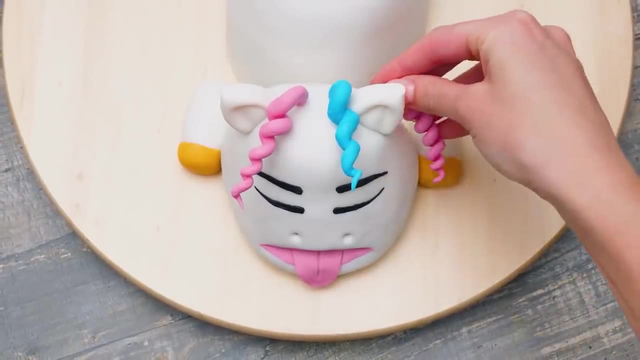 Can you help, Sure? First, let's put cute little ears in their place. And don't forget the curly mane. Uh, did I miss anything? The most important part: What is a unicorn without a magicorn? I was trying to trick you, Sammy. 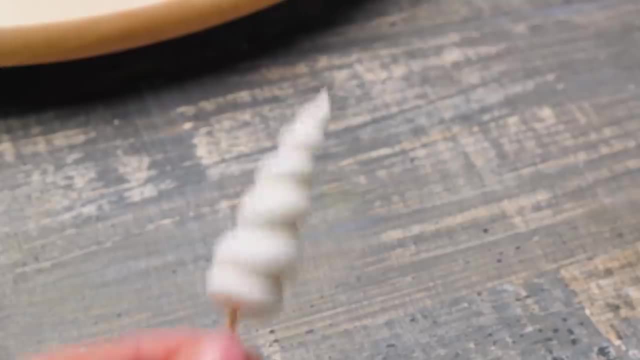 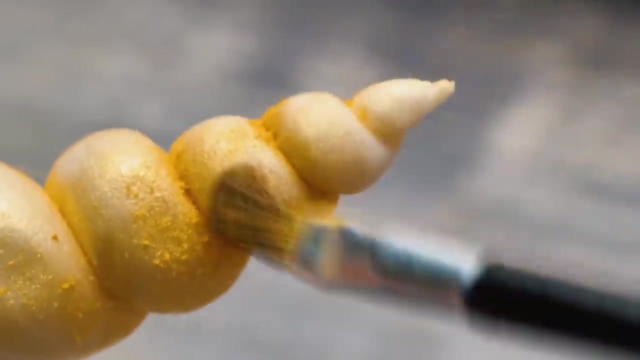 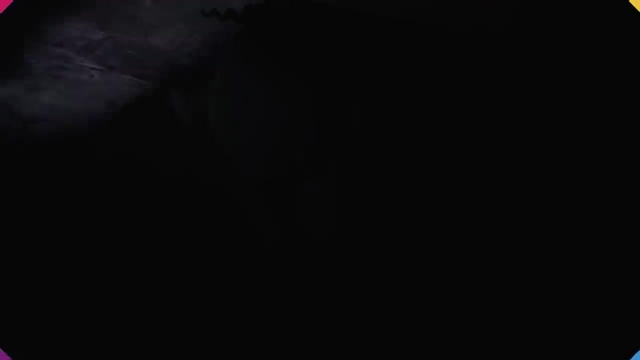 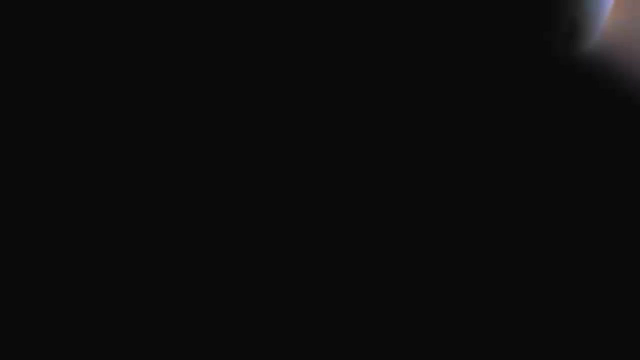 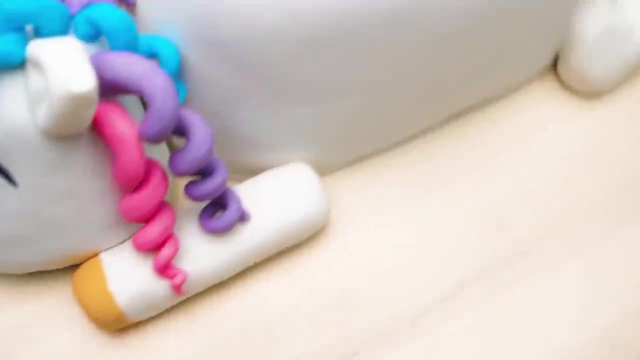 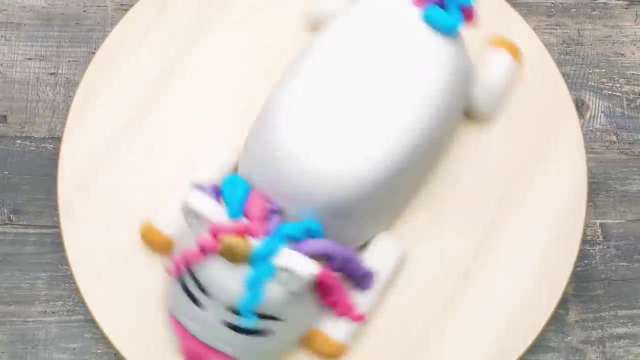 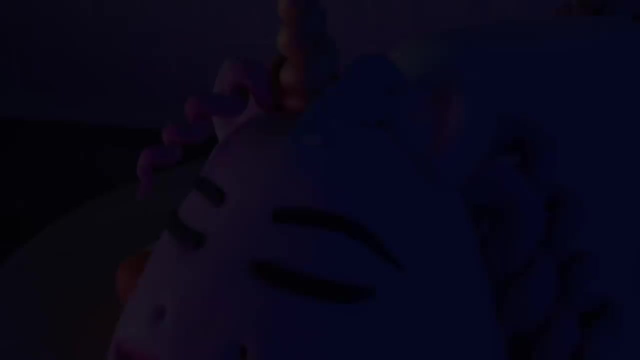 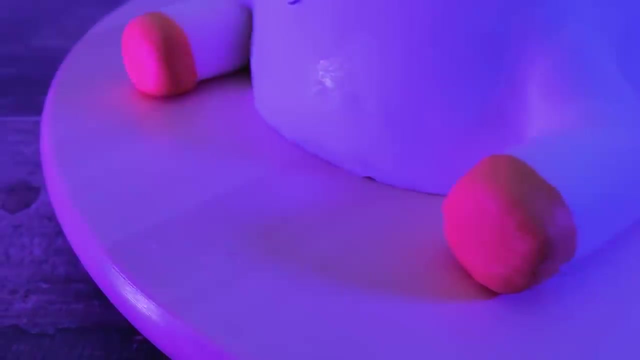 It's not a pony party, after all, is it? Now let's color it with gold glitter paint To highlight the magical background. Our amazing cake is finished. Let's enjoy the decor before the party. So pretty, It's so pretty. 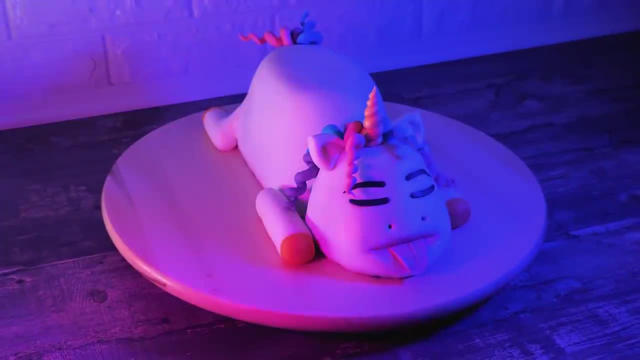 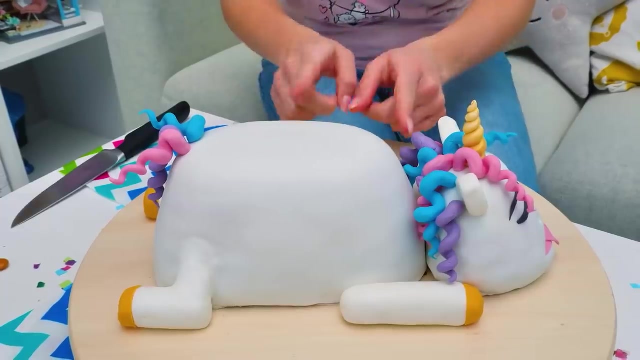 It goes down there. We need to add some colors in there. Can you guess what I'm going to put on my cake now? Holy-can-nolly, It's the best unicorn day, Sue. Yeah, And this cake is so pretty. 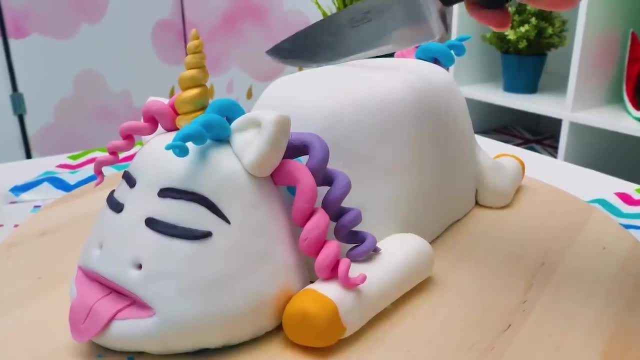 Not only from the outside, but from the inside too. This cake is beautiful to live in. Let's see how it looks. Let's dream, Let's dream. Guys, be very careful with the knife. I can't wait to see the result. 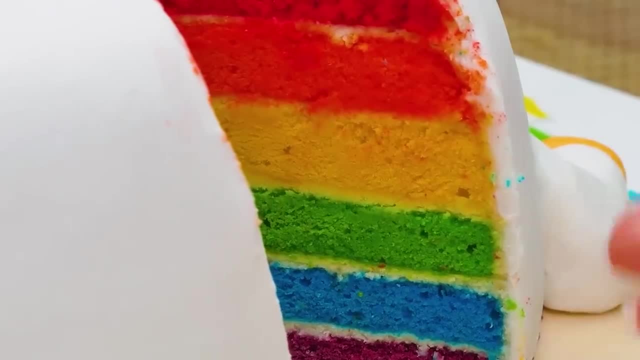 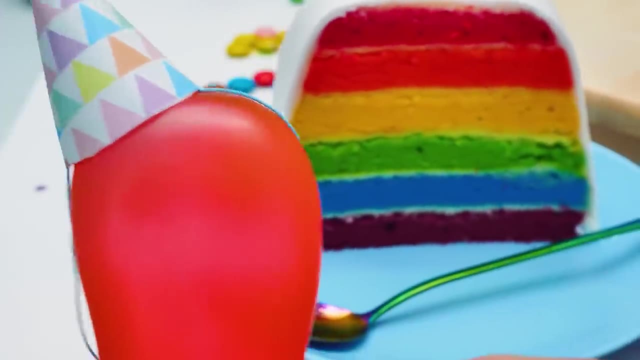 Wow, Check out these colorful layers. This is what cake was made for. Woohoo, Sue, I want a piece of a rainbow too. There you go: One piece for you and one for me. Sue, wait up, What were you talking about? 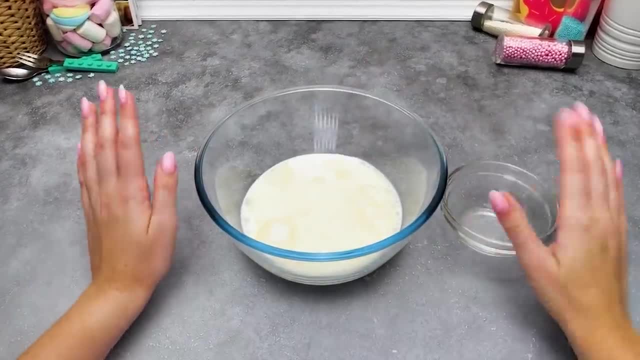 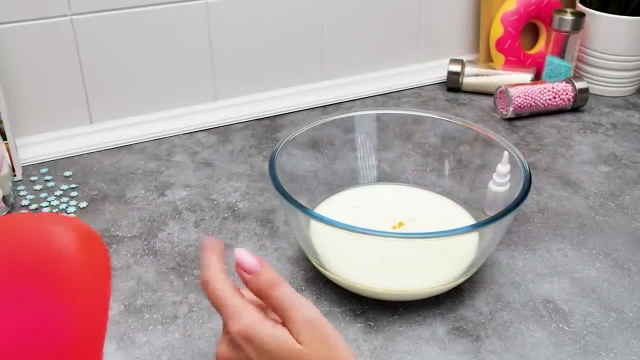 I was thinking: why don't we make a perfect Sam cake? Hi everyone, Susie, that's the best idea. Tell me everything. Well, this will be a combo of white cake and funfetti cake covered in tasty buttercream in the cutest shape of all. 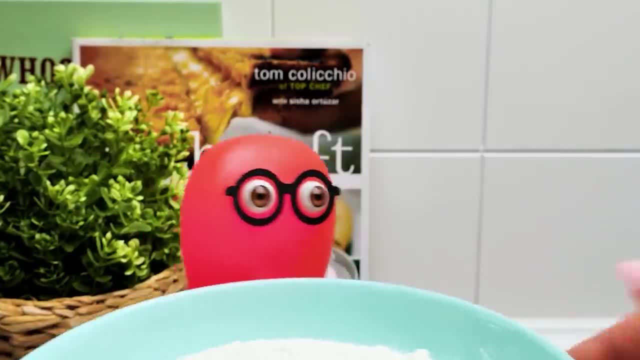 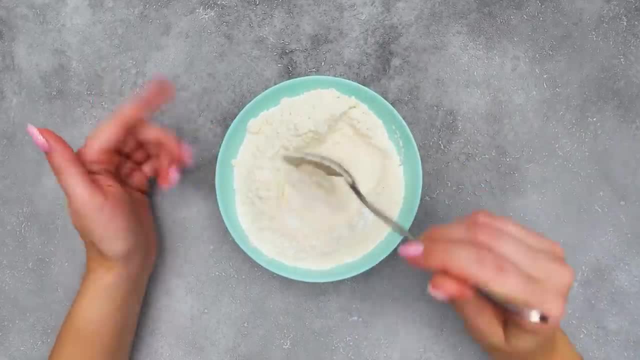 Yours. Huh, Awesome. In case you'll need a reference, I will be right there. No, no, no, mister. Oh, I actually want you to help me. Go and preheat the oven to 170 degrees Celsius. 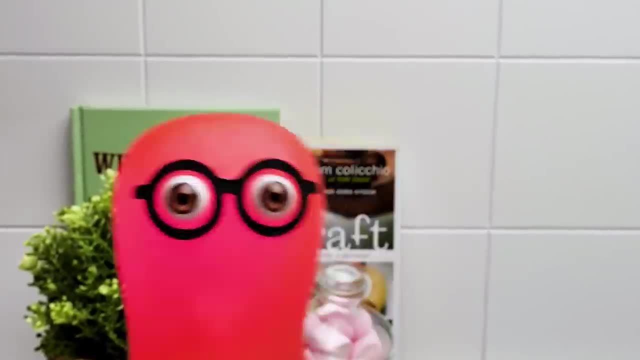 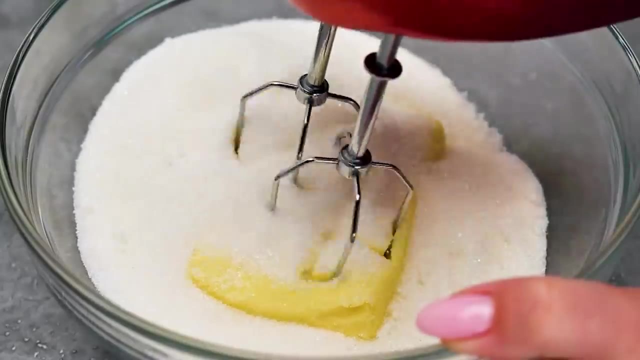 I'm a real pro at it, guys, but you should never use the oven without adult supervision. And while Sam's doing that, let's deal with the butter. guys, We need to mix it with sugar. really well, Here we go. 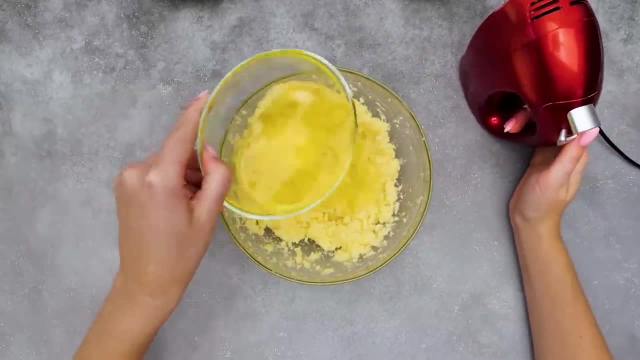 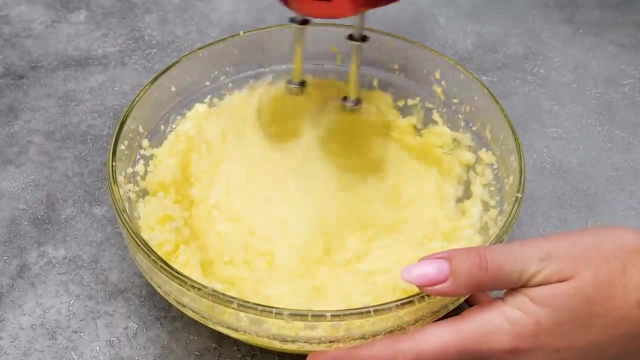 Now it's time for the egg whites. It's really important for them to be at room temperature. Actually, all of the ingredients had better be at room temperature, Otherwise you could get a fallen cake. Susan, the oven is ready as well as I am. 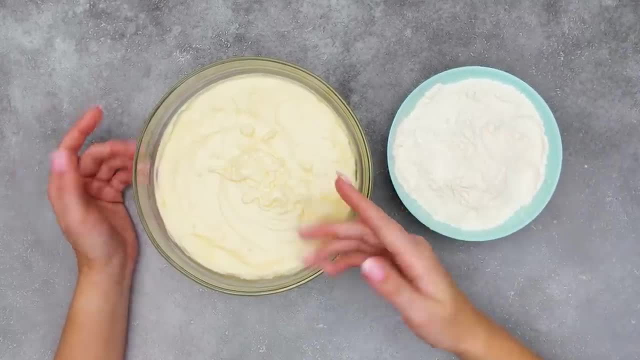 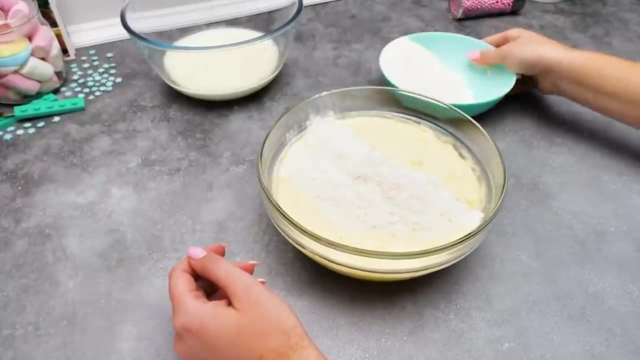 Oh, somebody dressed up. Well, we're almost done with the butter mixture. Now we need to combine it with our dry ingredients: flour, baking powder and salt. Great memory, Sammy. But we'll do it gradually, in three even parts. 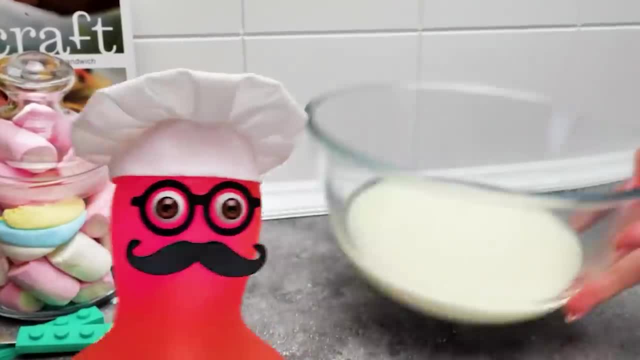 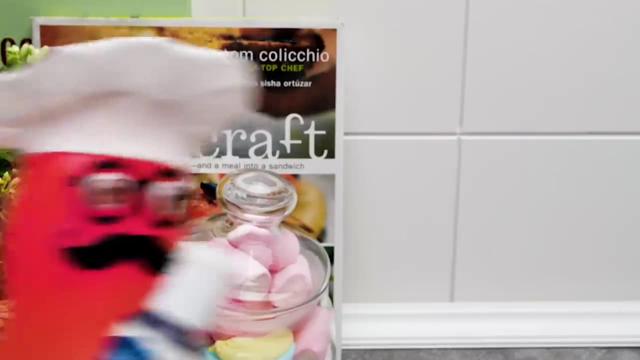 And in between those, we'll be adding our liquids, milk oil and extracts. Susie, I've been thinking: even though this cake is called white, why don't we make it pink? That's the same cake, after all, and I can hardly be called white. 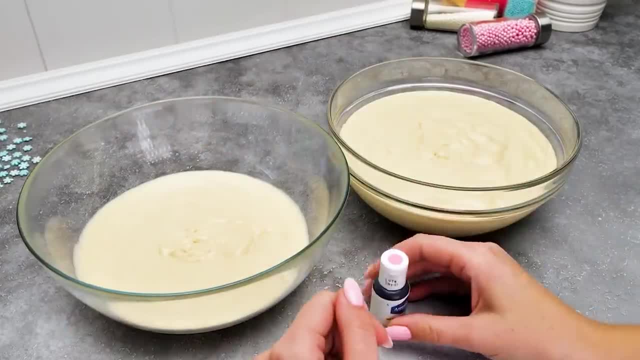 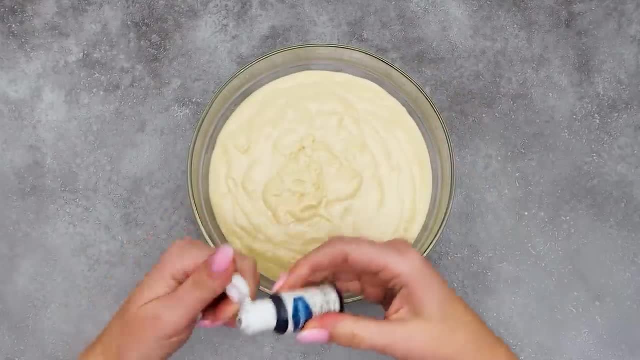 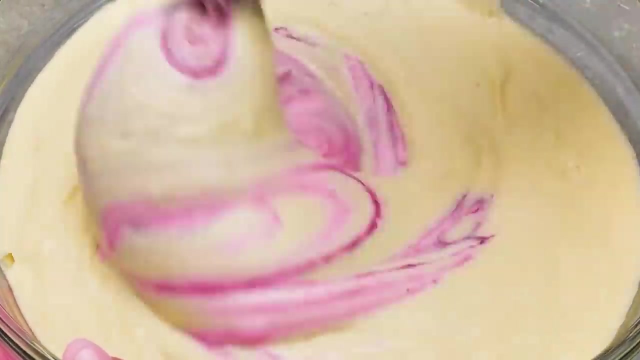 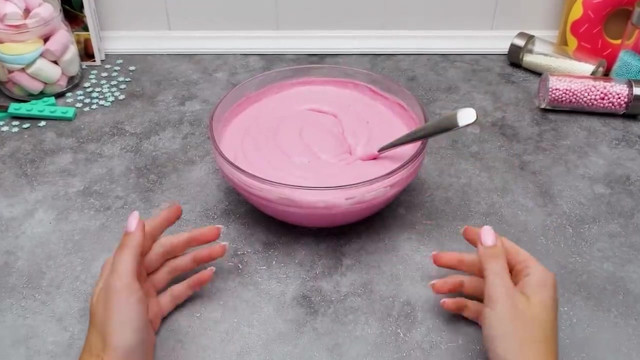 You know, that actually is a great idea. We will leave it at room temperature. We will use this batter for both types of our sponge cakes. This part is to be colored pink. Here we go. All we've left to do is to divide this batter into two parts. 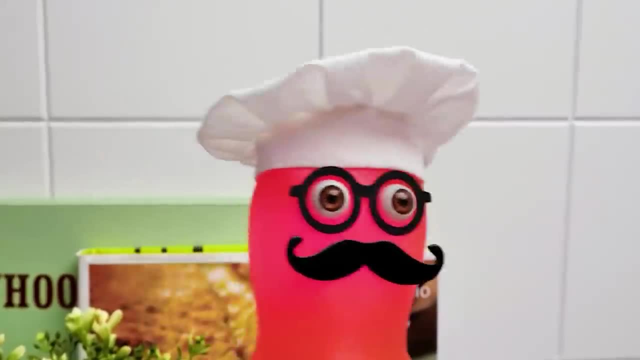 Oof, I'm gonna go take everything to the oven, But come back quickly, Sammy, cause we're gonna deal with the sprinkles. I'm gonna go take everything to the oven, But come back quickly, Sammy, cause we're gonna deal with the sprinkles. 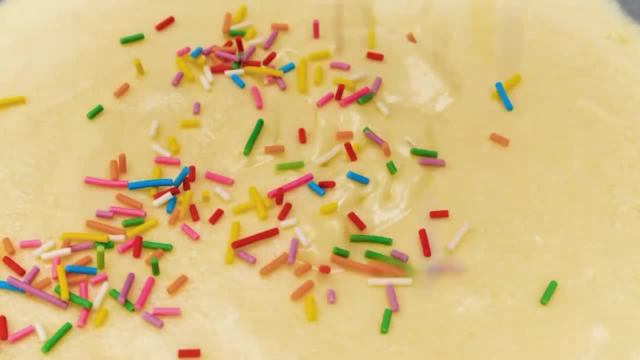 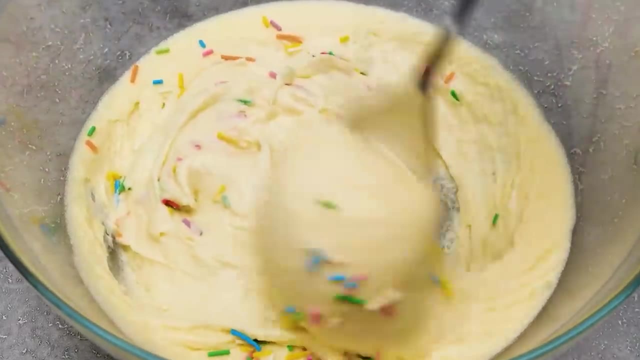 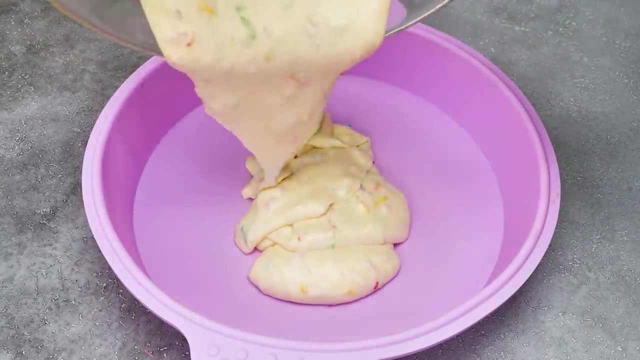 Here we go Carefully. Now we'll mix it really well so the sprinkles spread out evenly. The final step is to pour the batter into the mold. It looks awesome, am I right, guys? Did I miss everything? No, Sammy. 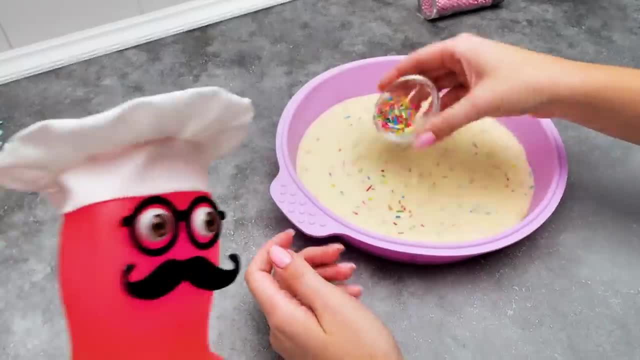 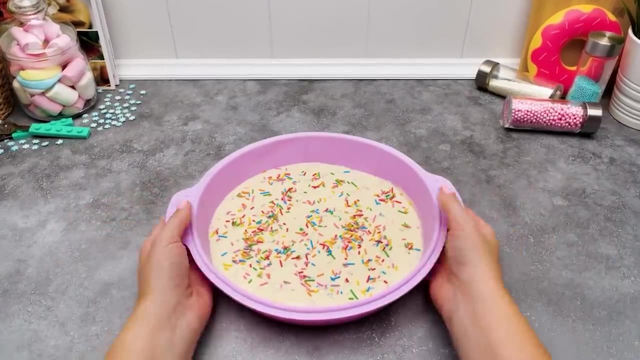 We're about to add some more sprinkles on the very top, Like this: Wow, Okay, Then we're going to bake all our future sponge cakes for 30 to 35 minutes and then cool them. Stay tuned, guys. The best part is yet to come. 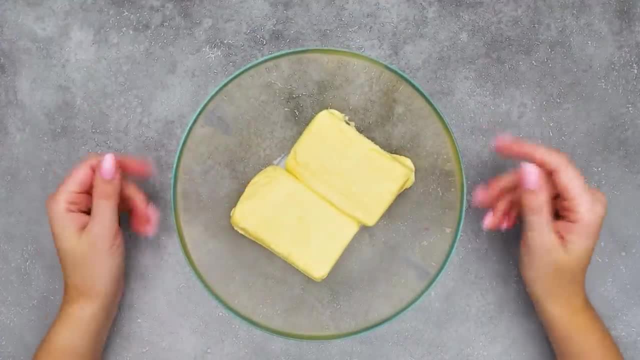 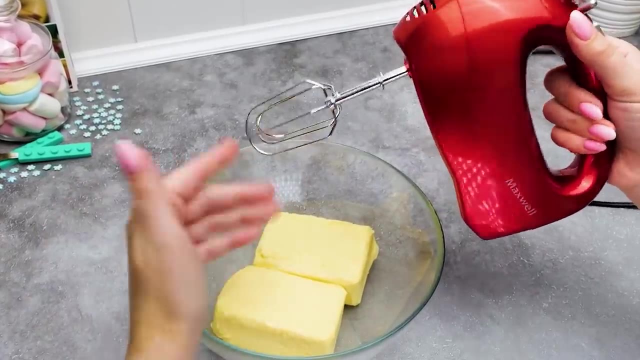 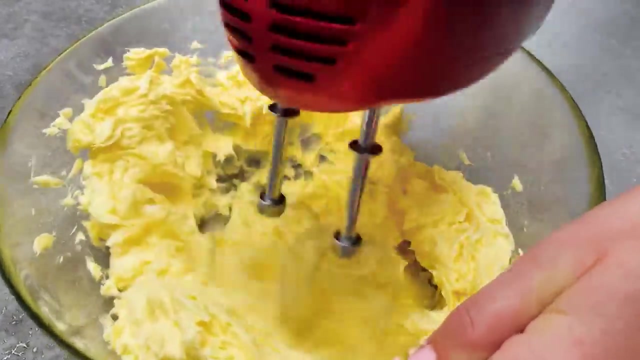 While our sponge cakes are cooling down, let's make the buttercream. Here we have 340 grams of softened butter. We're going to whisk it really well till it has a nice fluffy consistency. And here's the powdered sugar. I'd like to call it sweet snowflakes. 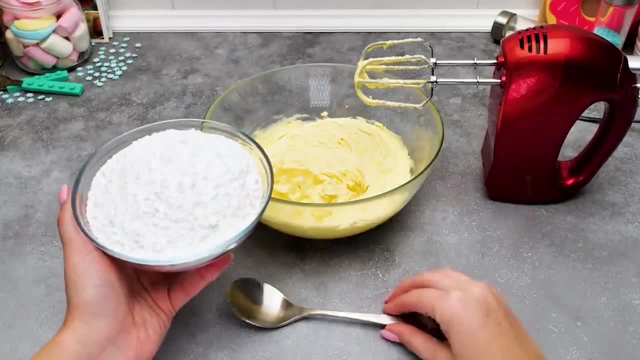 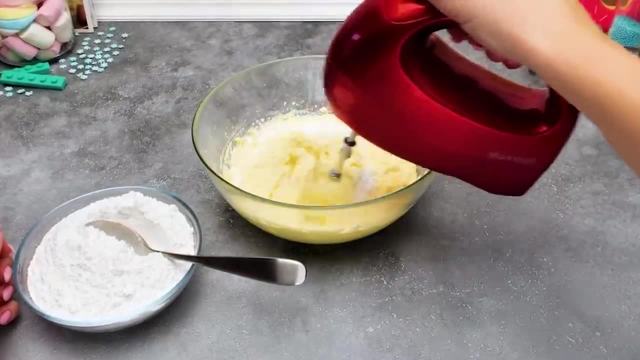 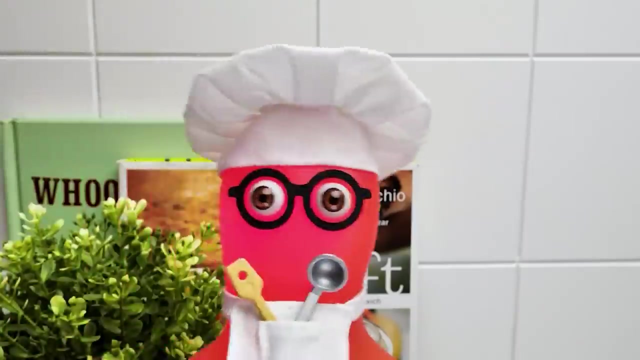 Sammy and his imagination. We need to combine these ingredients really well. until we get a uniform structure, We'll just add one spoonful followed by another. So yeah, it's kind of a slow and steady process. Here's a quick tip for you from Chef Samuel. 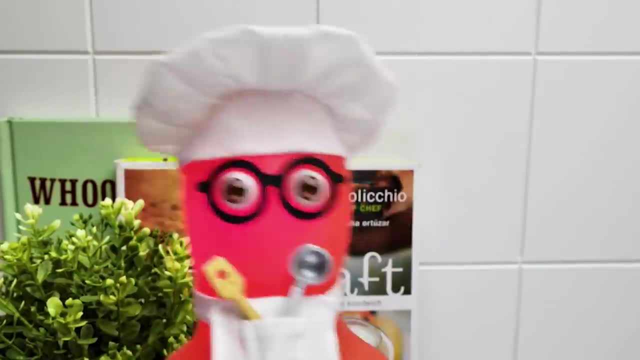 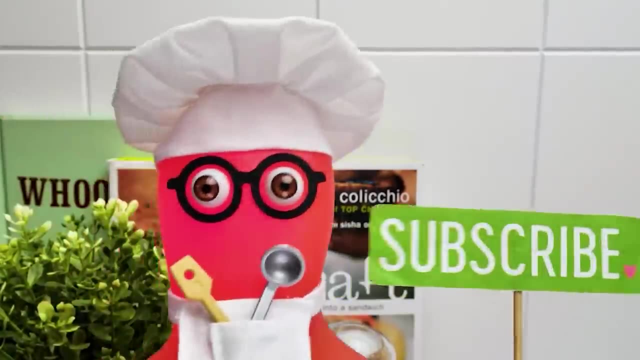 Sift your powdered sugar. Sift your powdered sugar beforehand. This way, your buttercream will incorporate all the air and become really fluffy. By the way, guys, if you like cooking with us, give us a thumbs up and subscribe to our channel. 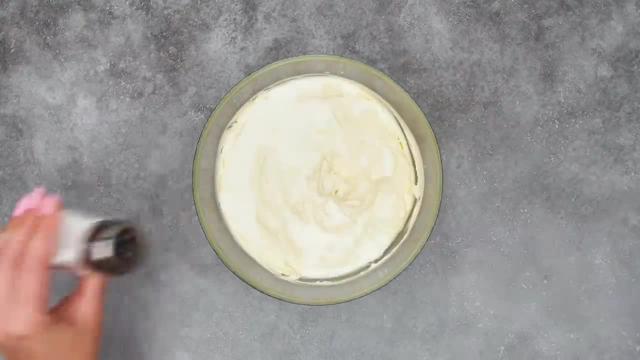 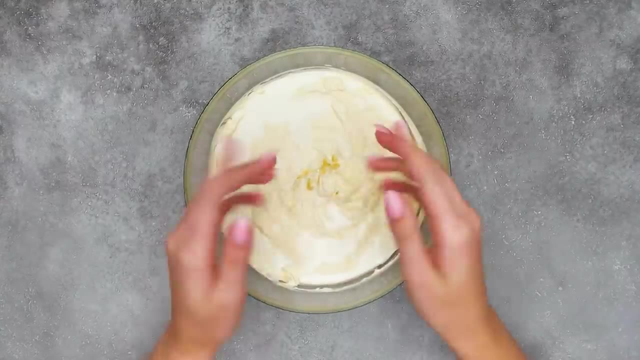 Okay, now we'll add just a tiny bit of milk, a pinch of salt and a few drops of vanilla extract to enrich the taste of the buttercream. But plain white is not exactly what we need. Let's color it this way. 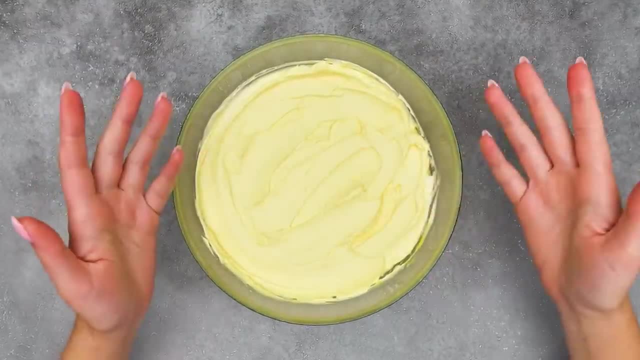 Check out this amazing look. Ooh, it smells so good. So what now, Susie? Are we ready to assemble my cake? Don't rush, Sammy. The preparation stage is very important in cooking. Besides, we want your cake to be really special. 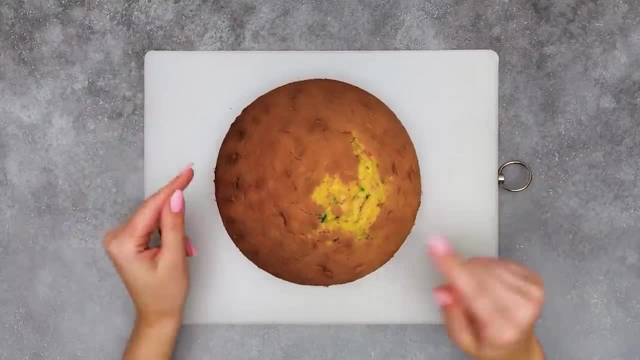 Wow, Sue, is that a Funfetti sponge cake? Right you are. We need to trim it a bit to make it look even. We need to do the same with all our sponge cakes. Mmm, this looks delicious. Guys, Sue and I are going to finish here. 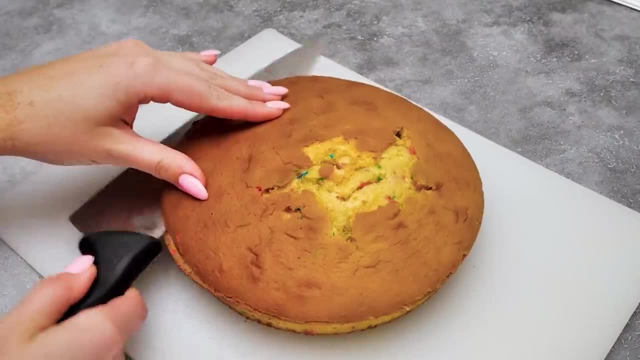 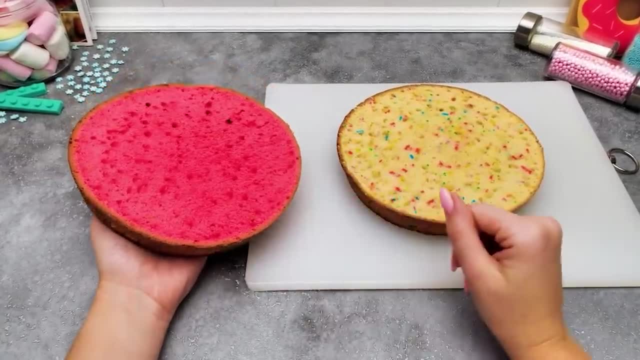 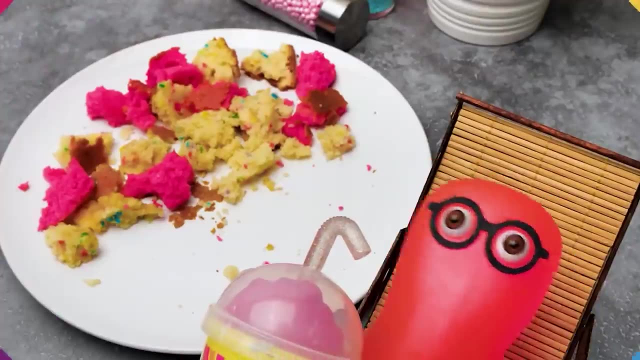 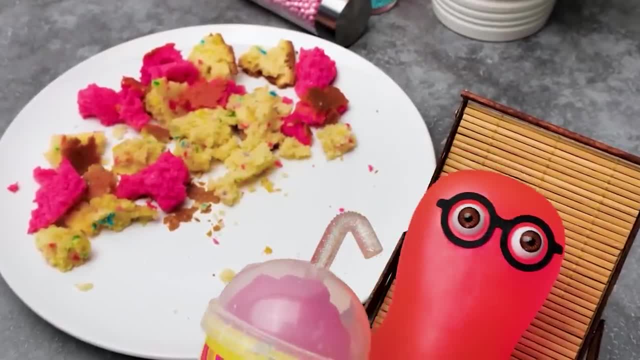 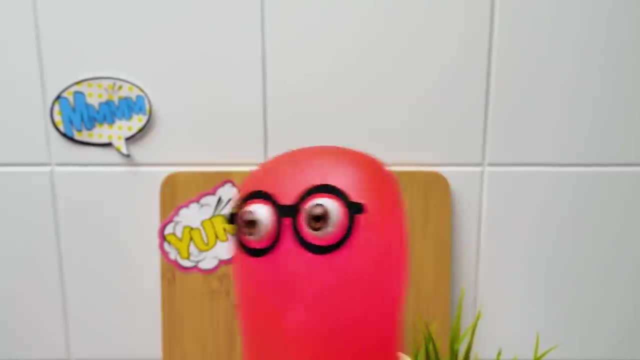 I'm so excited. I'm so excited. Ah, Okay, guys, now we'll need a cardboard circle. Wait, what? Like this one which is cut out of the cake board? See Ahem, Suzie, don't you think that you've messed up two crafts? 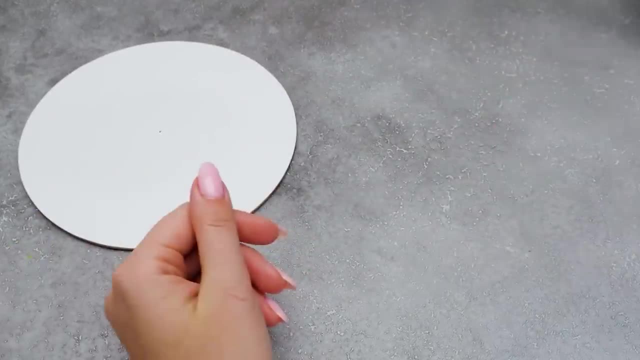 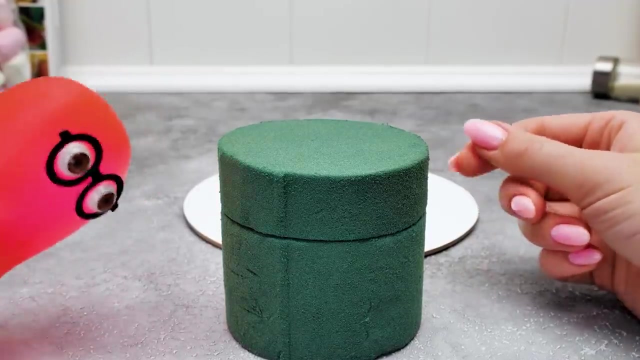 Well, actually we'll be using quite an extraordinary prop today. Check this out. This is a piece of craft foam that you can buy in any craft store. Is it edible? Of course not. Sammy will serve as the base for our cake, But since it will be touching food, let's cover this. 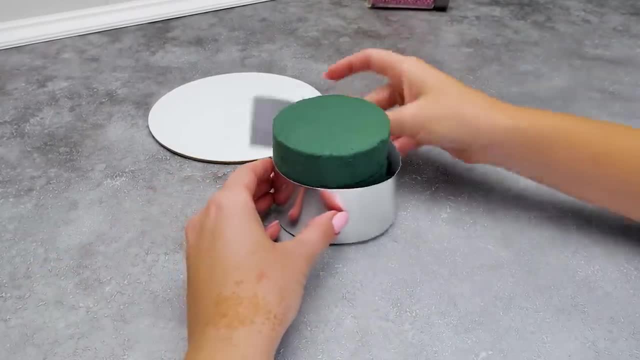 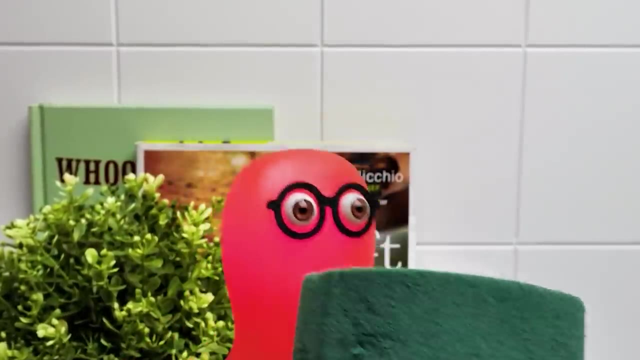 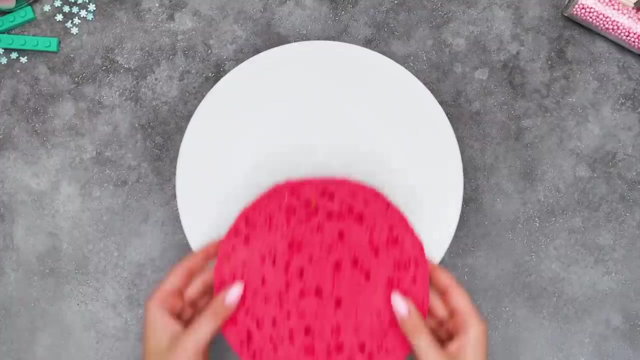 piece with aluminum foil tape. Let me deal with it, Sue. Now I'm really interested in what's going to happen next. Ha ha ha. Okay, in the meantime, guys, we'll start assembling our cake. We'll defo need this thing. We used some buttercream to make the cardboard. 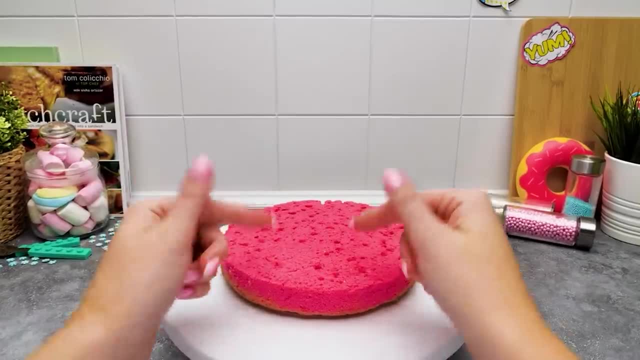 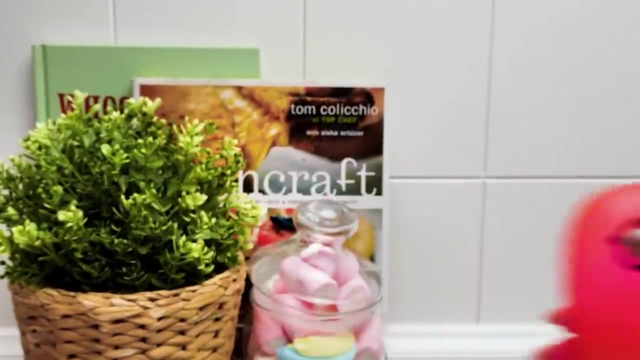 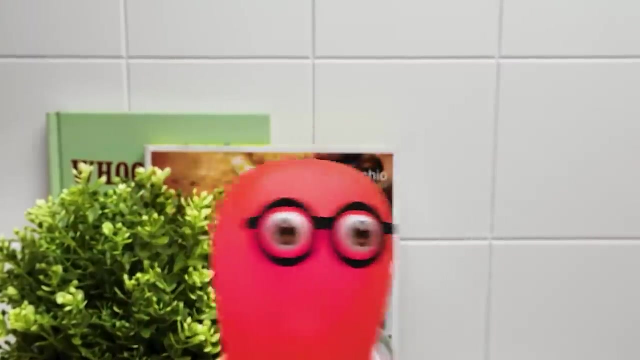 piece stick to the sponge cake. And now we simply need to layer all of our sponge cakes with the buttercream. There we go Right on time. Whoa, Now please stand still. It's time to give our cake its shape. Susie, are you sure you have a steady hand? I'm kind. 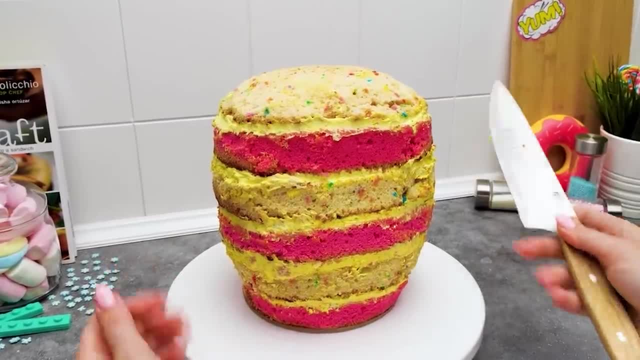 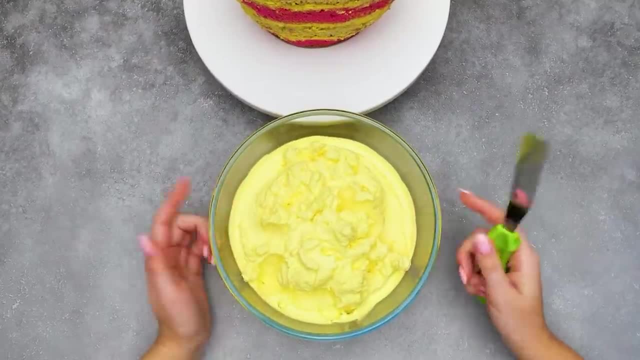 of worried. Don't move, Sammy, It's almost done. Excellent, Wow, Holy cannoli, That looks more like a balloon. Don't worry, Sammy, We haven't finished yet. We gotta cover our cake with a thin layer of buttercream all the way around. This is called crumb coating. 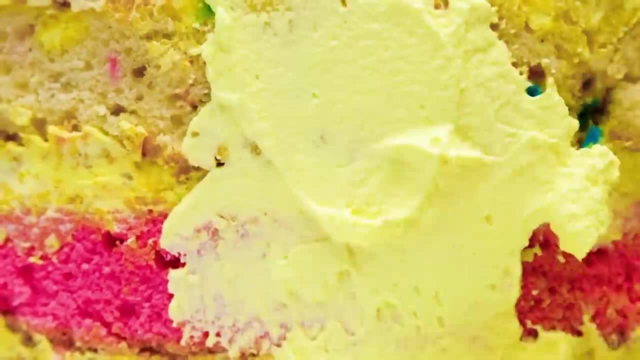 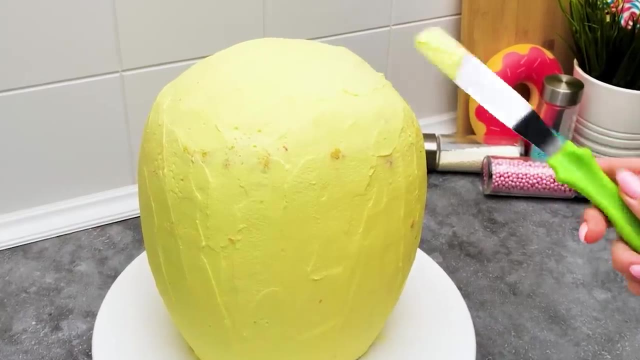 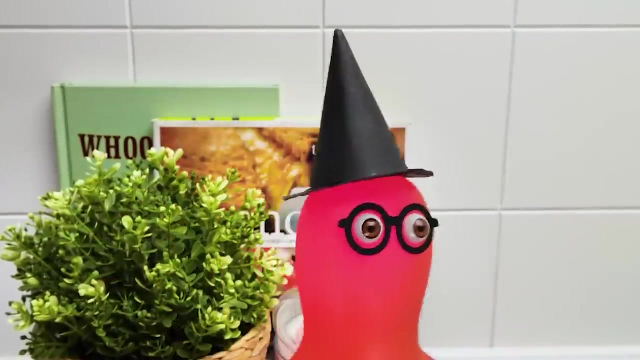 And a couple more touches. Perfect Guys, we need to let this buttercream freeze properly, and I'm gonna use some magic Hold it, But now, Actually, we've still got plenty of stuff to do and we'll need your freezing magic later. In the meantime, let's take our cake. 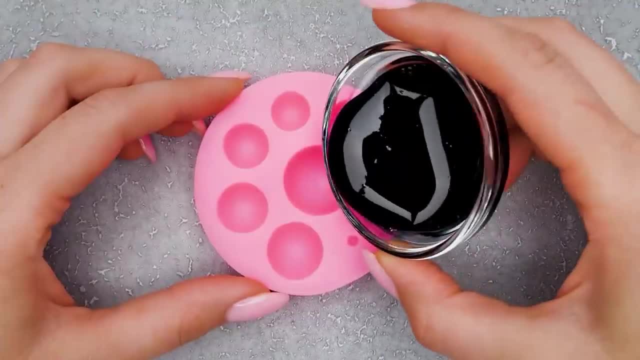 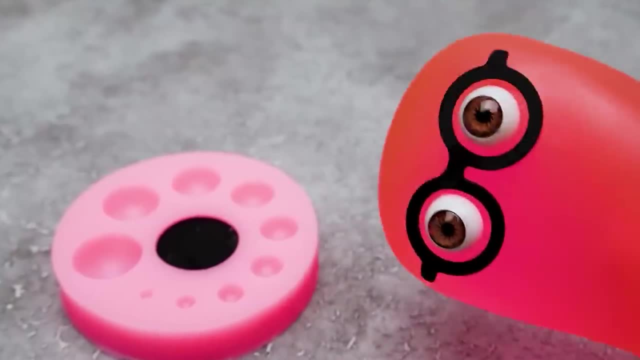 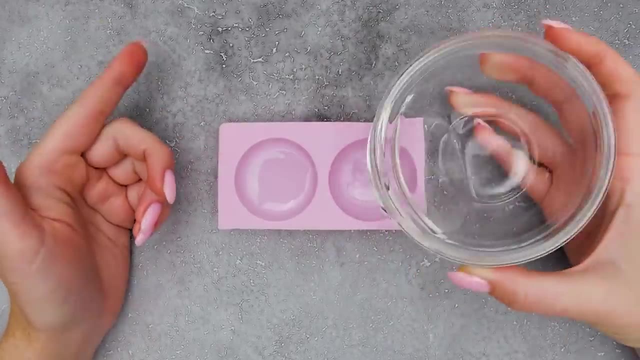 mm-hmm, mm-hmm, mm-hmm, mm-hmm. Is this chocolate, Susie? Nope, This is called isomalt, something like a candy. We're right in the process of making edible eyes for our cake, And now we can place our black pupils. 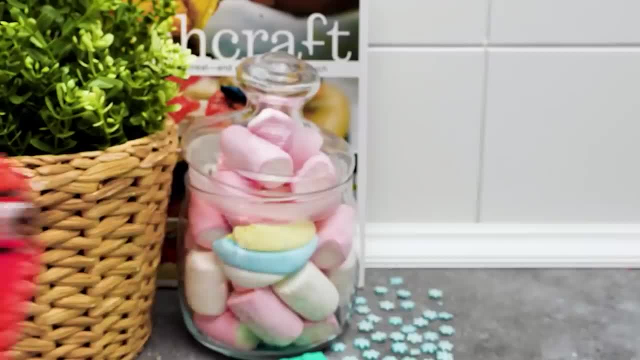 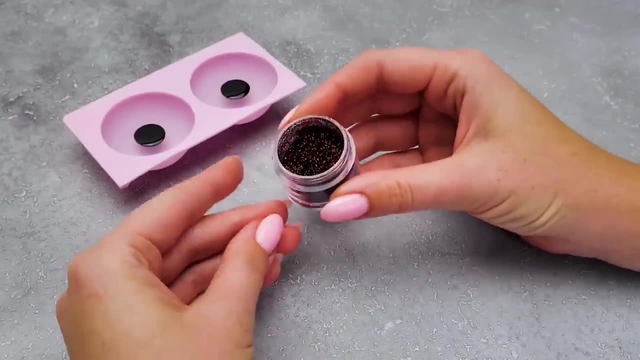 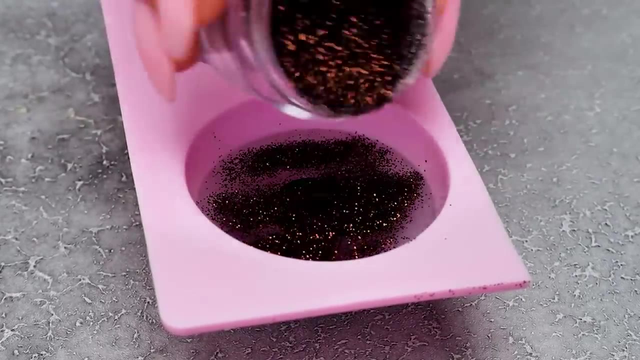 straight in the center of these eyes. Whoop, How cool is that? Give us a thumbs up if you agree everybody. Here comes the really sparkly part of our cake: cake gloss. We chose this color because Sammy's eyes are beautifully brown, Doesn't it look magical? 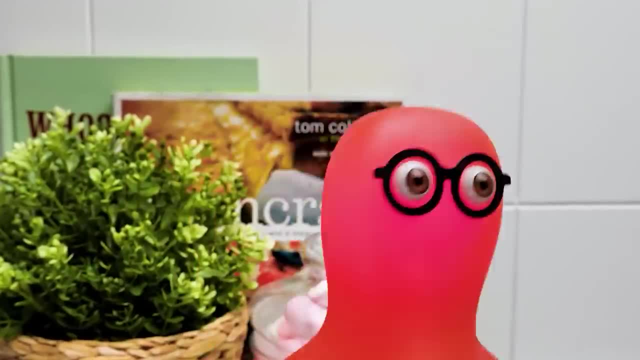 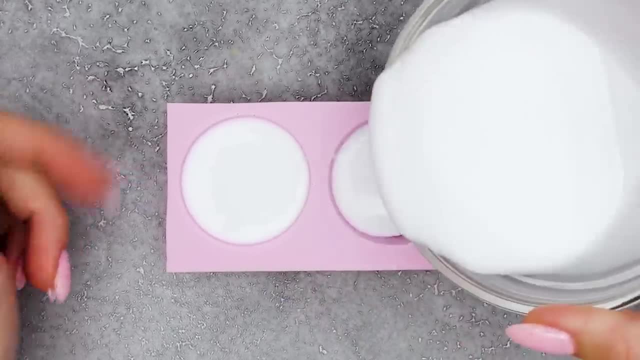 Let me help you, Susie, or we'll never finish today. Sure, Sammy, Just let me finish with the white isomalt here. Great Looks good, And now we can leave this thing aside to let it cool and work with the fondant to make a nice base. 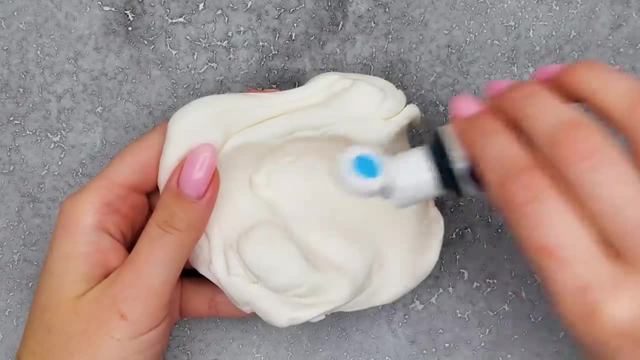 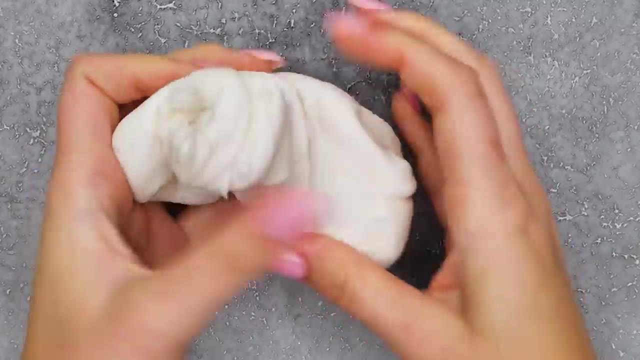 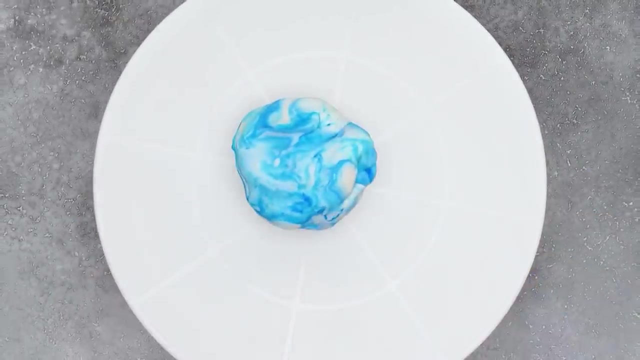 for our cake. We'll add just a little bit of this magical blue food coloring to make this fondant look spectacular. Susan, help me. Oh, well done, Sammy. Thanks, I'm going to show you a little trick, guys. Here we go And voila, Our cake board is ready. 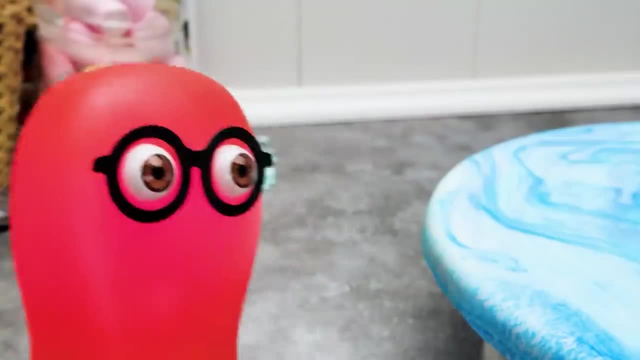 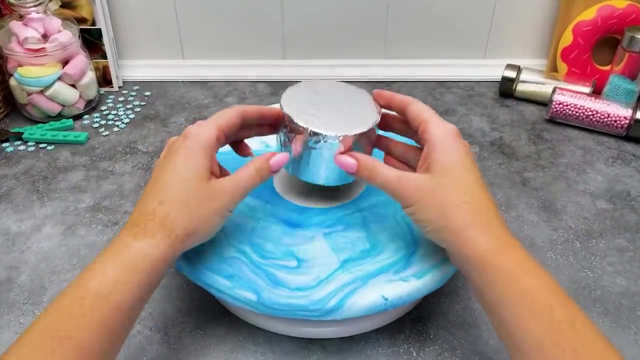 now We just have to cut a circle in the center. I don't get it, Sue. We're working and working, but I still don't see the cake. Give me a few more seconds Now. we can place this thingy right here. 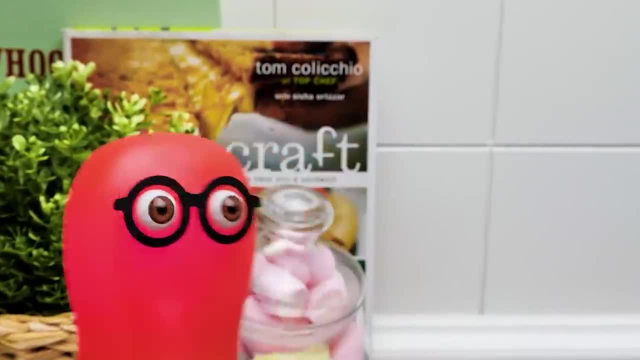 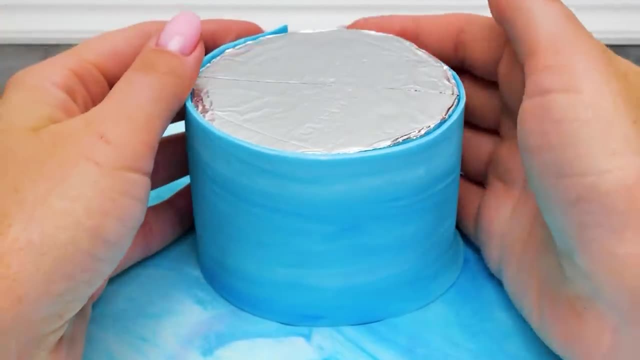 Shiver me cheddars. Sue, you were right earlier. We are totally using strange tools for a cooking craft today. Oh, by the way, Sammy, remember our cake part. It would be nice if you were able to do it yourself. 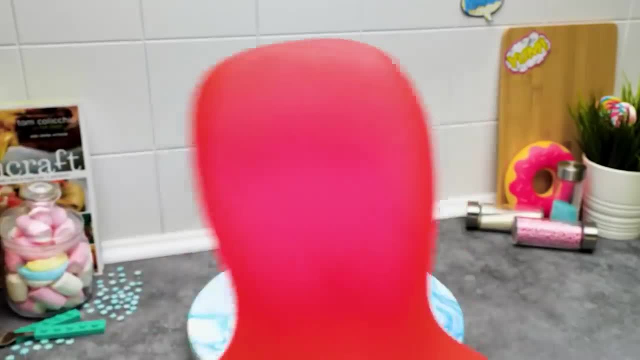 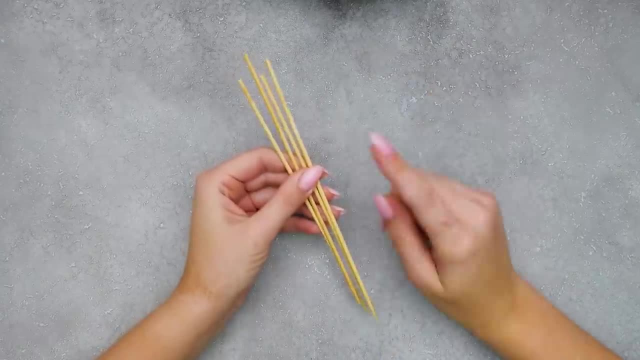 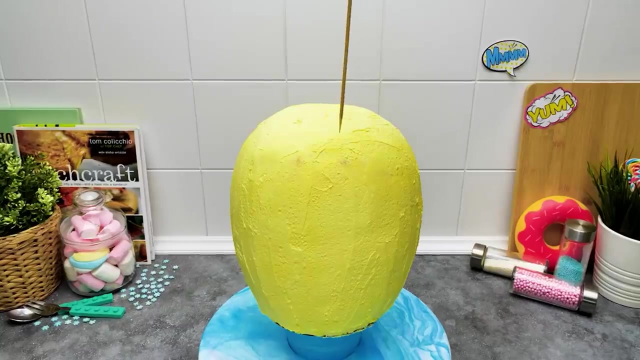 It would be nice if you brought it here. I'm on it. Easy, There you go, Sue Terrific. Now, just to make sure that nothing's going to fall apart, let's insert skewers all the way down to the cake board, like this. And the last one: 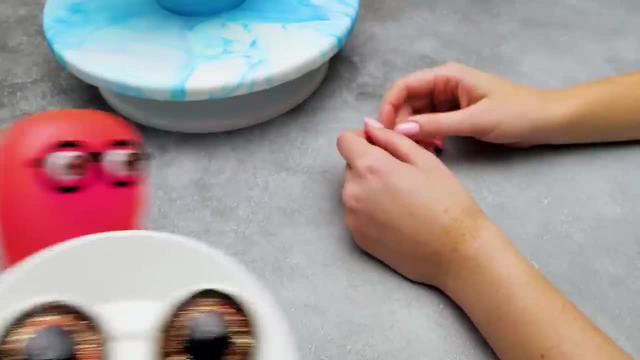 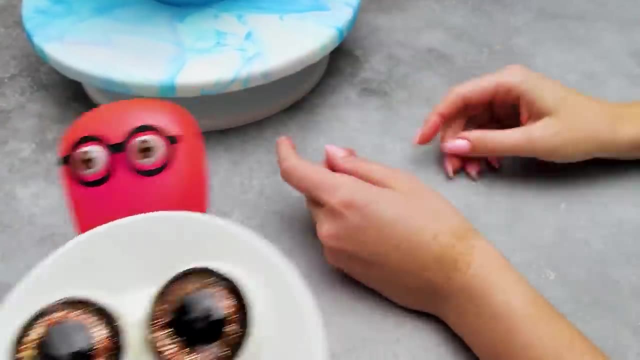 Oh, wow, What happened, Sammy Susie? I removed the ice from the mold and they're really sparkly. Check them out. Wow, You're right, They look awesome. Let's finally cover the whole thing with pink fondant. 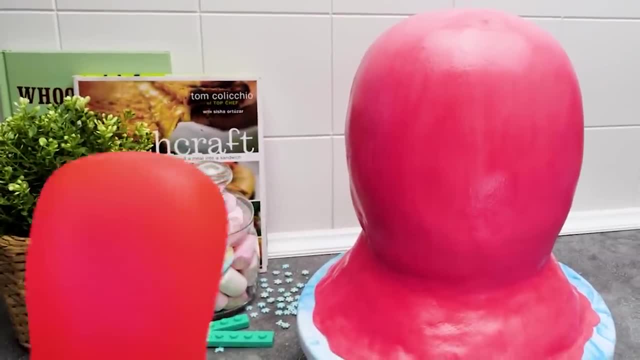 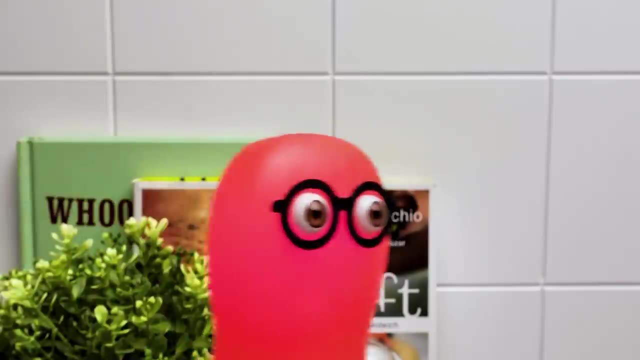 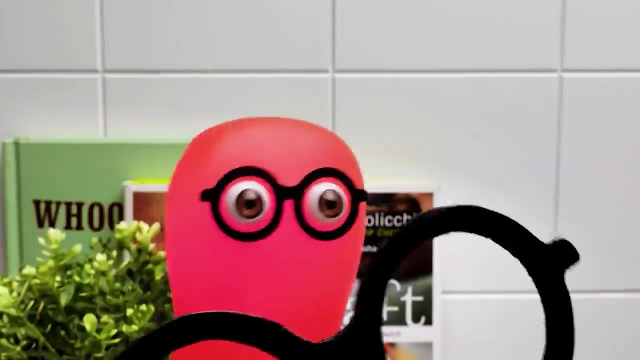 Wow, I'm so big And, pretty sure, very tasty. Sammy, check this out. Ta-da. Wow, he looks just like me, But one thing's missing. What is it? Oh, I know Here They're too big for me anyway.